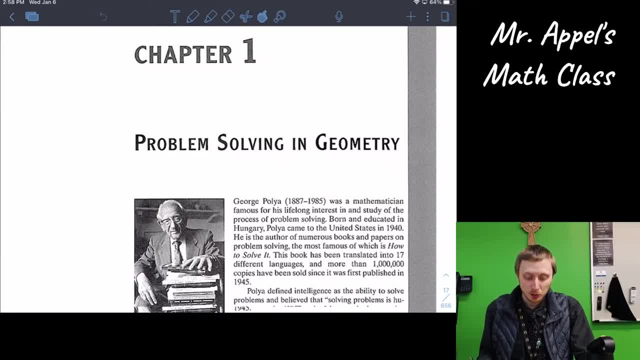 Hello and welcome to a read-along for College Geometry: a problem-solving approach. Today we'll be going through reading, highlighting and annotating Chapter 1, Problem Solving in Geometry, specifically Section 1.. We'll begin here with a bit of background information on a man named George Paglia. 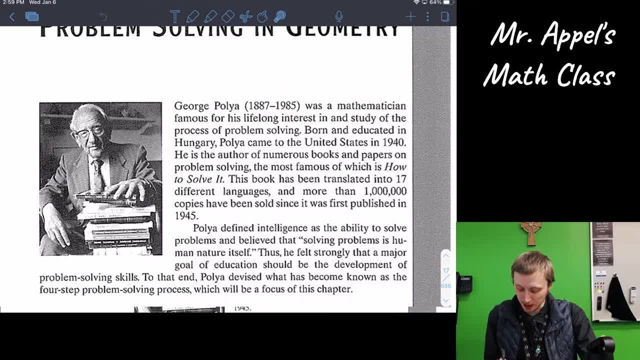 born 1887, lived to 1985.. He was a mathematician famous for his lifelong interest in, and study of, the process of problem-solving. Born and educated in Hungary, Paglia came to the United States in 1940.. He is the author of numerous books and papers on problem-solving, the most famous of 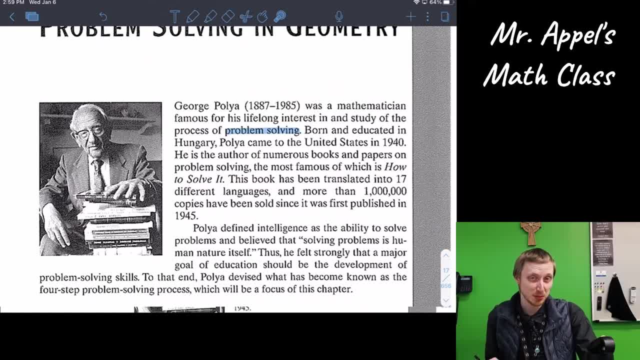 which is the book The Problem Solving. He is the author of the book The Problem Solving, which is How to Solve It. I've looked at that book. I would not say it stands the test of time. It's kind of a difficult read for modern standards. This book has been translated into 17 different 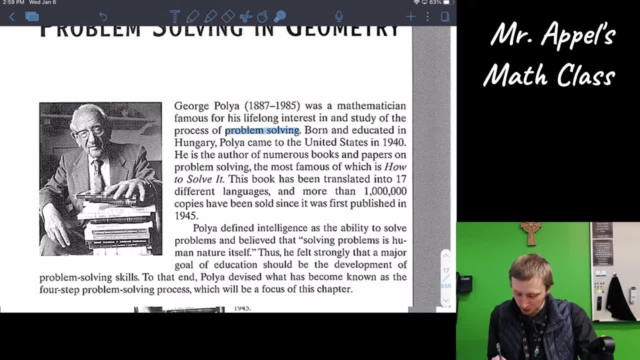 languages and more than 1 million copies have been sold since it was first published in 1945.. The foundations, though the ideas in that book, however, are fantastic and incredibly useful. Paglia defines the problem-solving as a problem-solving approach. He says: 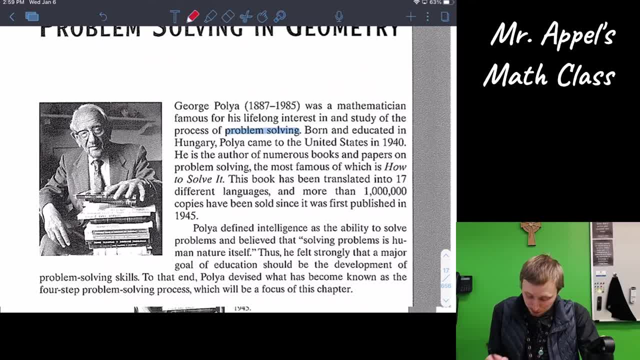 Paglia defined intelligence as the ability to solve problems. Intelligence is the ability to solve problems, And I think a lot of intelligence tests are based on that very concept. Believed that solving problems is human nature itself. That's a powerful thought. Thus he felt strongly that a major goal of education should be the development of. 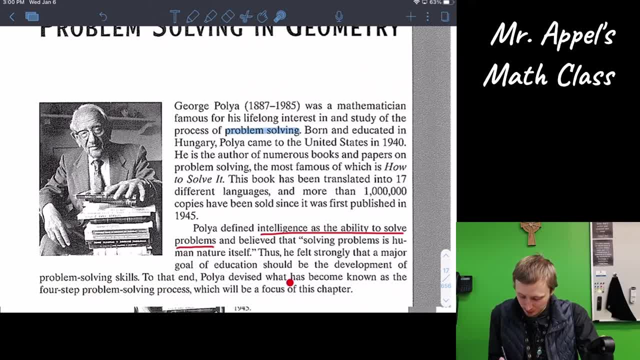 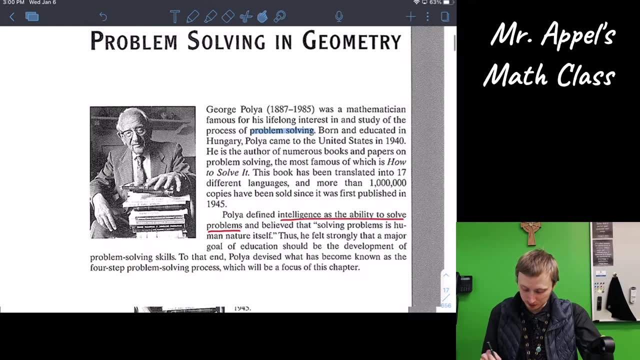 problem-solving skills. To that end, Paglia devised what has become known as the force step problem-solving process, which will be a focus of this chapter, That entire idea of which is the reason for this very video. Let's go on. Chapter 1, Problem Solving in Geometry. 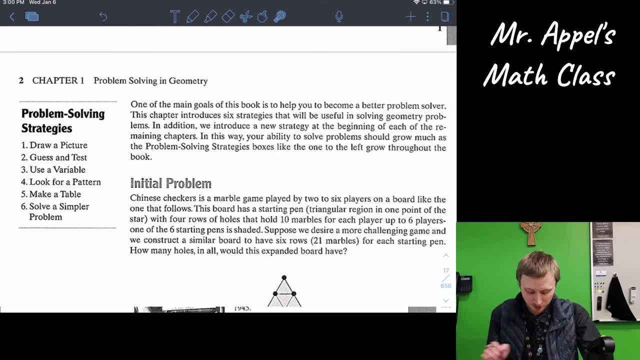 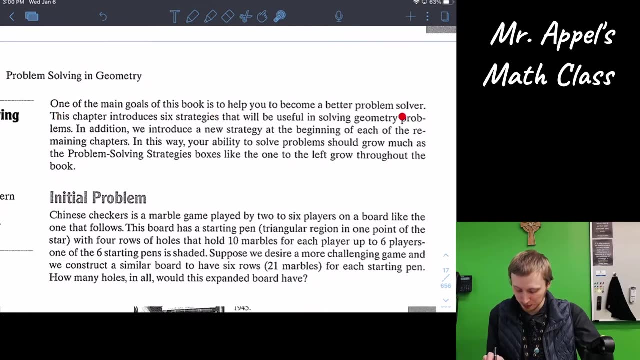 We have our listing of the first six problem-solving strategies there on the left and an initial problem to look at below. Let's start with the introduction. One of the main goals of this book is to help you become a better problem solver. This chapter introduces six strategies that will be useful. 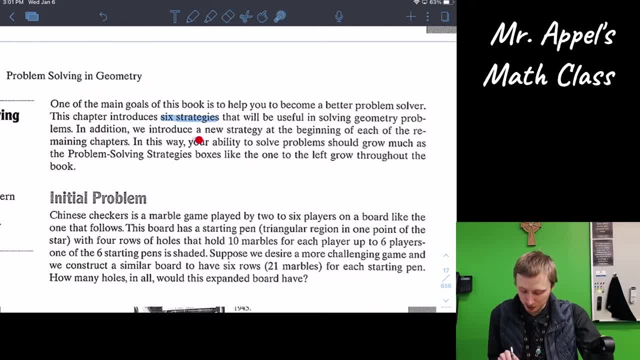 in solving geometry problems. In addition, we introduce a new strategy at the beginning of each of the remaining chapters. In this way, your ability to solve problems should grow much as the problem-solving strategies boxes, like the one to the left, grow throughout. 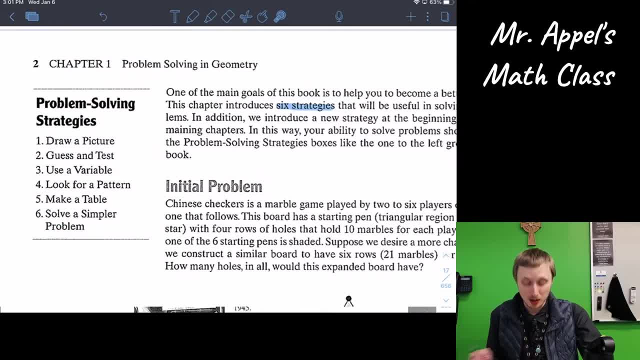 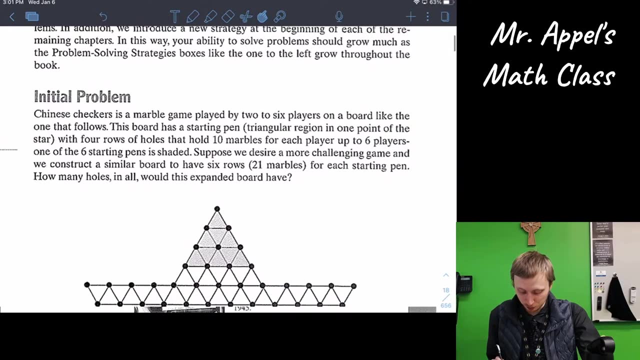 the book. So there you go. If you have this book yourself and you want to spoil it for yourself, go ahead and scroll down to that last chapter and take a look at how this list has expanded One initial problem. It says a problem, so I'm guessing you can use some of these strategies. 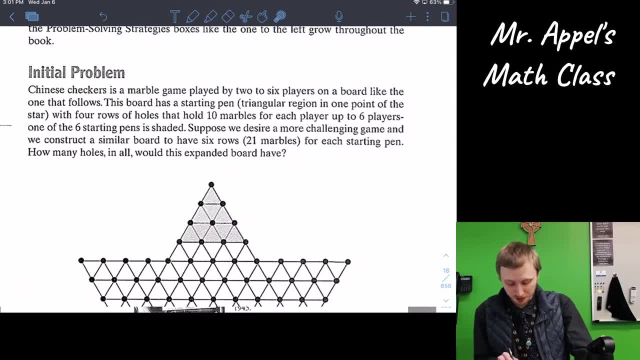 on this. Chinese Checkers is a marble game played by two to six players on a board like the one that follows. This board has a starting pen, triangular regions at one point of the star highlighted here, with four rows of holes that hold 10 marbles: One, two, three, four. 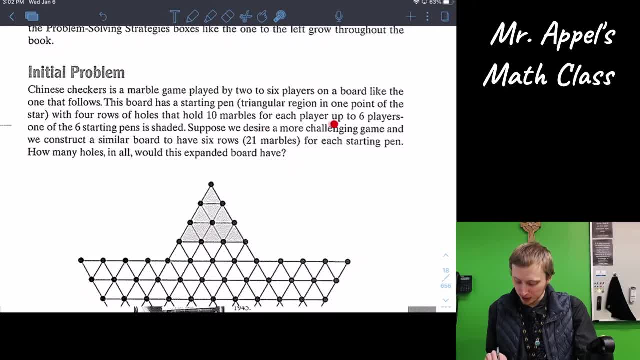 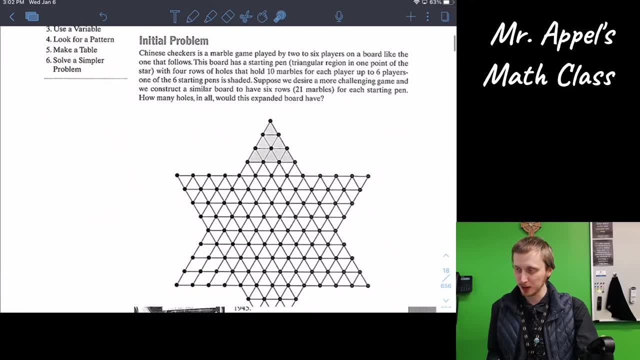 five, six, seven, eight, nine, ten. there we go, For each player, up to six players. one of the six starting pens is shaded right and I'll just zoom out so you can see the whole picture there. Okay, so here suppose we load buttons on top of this first right, And this is where 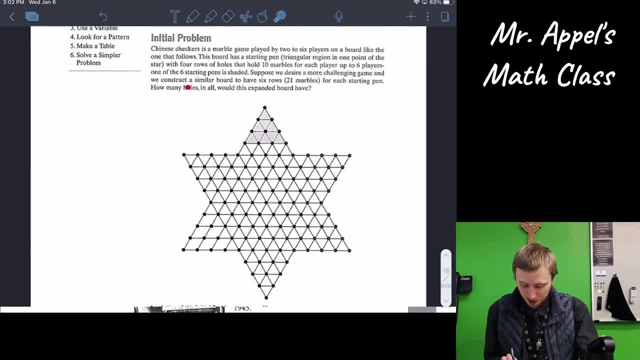 we take our board Here. we take our board by pressing the stops button. you'll see something. We desire, a more challenging game, and we construct a similar board to have six rows, 21 marbles for each starting pen. How many holes in all would this expanded board have? 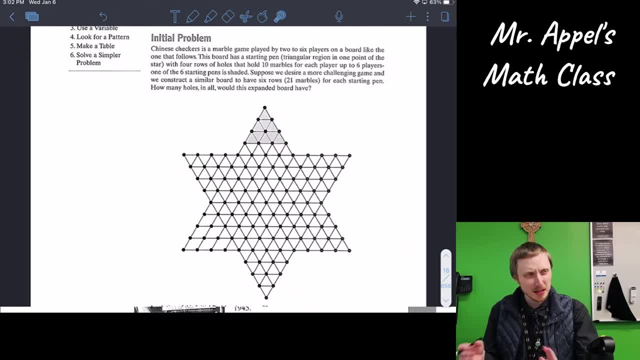 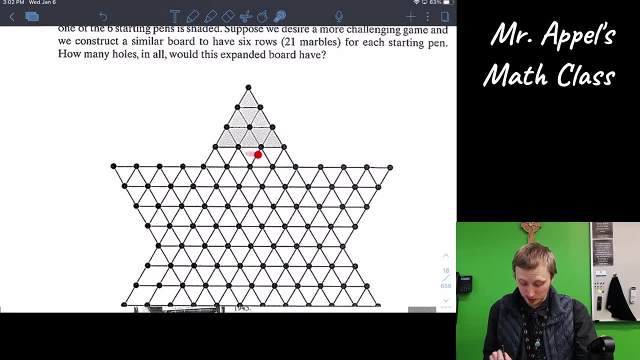 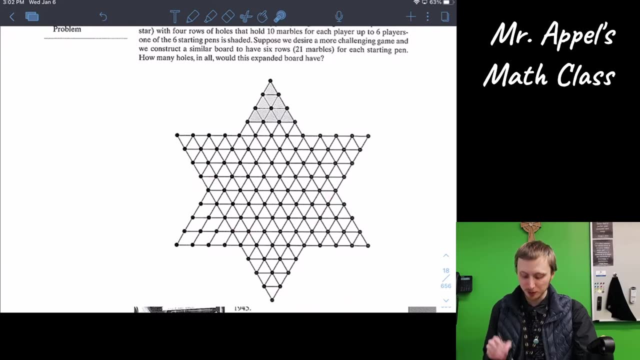 Go ahead and pause the video here for a moment and think about that for a bit. What would that entail? What would the starting pen itself look like? Keep in mind that you'd have six of them. What would this middle section between all the pens have to look like in order to make? 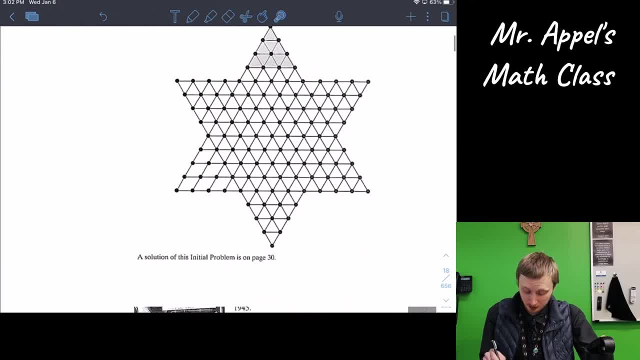 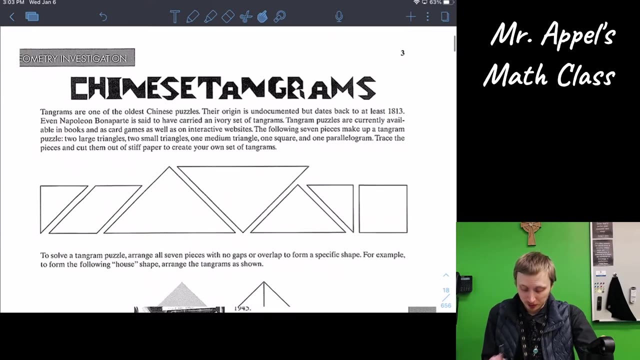 that work. A solution of the initial problem is on page 30. Unfortunately, that's the end of the chapter. after section two, You'll have to wait until the next video to see the solution. And before we get into the text, each chapter also opens with an investigation- a fun activity. 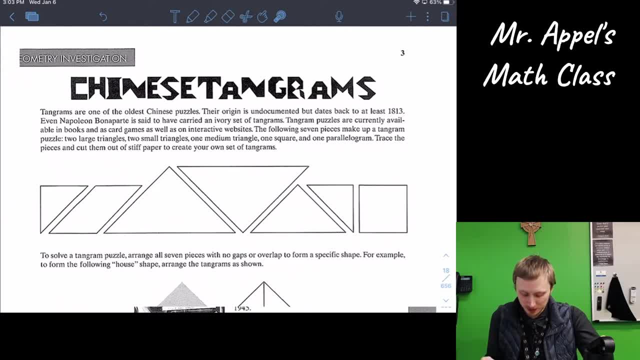 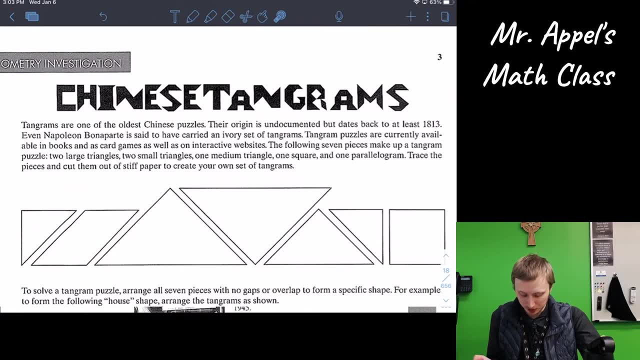 to get your brain and fingers working. This one introduces Chinese tangrams. Many people have played these in their childhood. I'm sure Tangrams are one of the oldest Chinese puzzles. Their origin is undocumented but dates back to at least 1813. 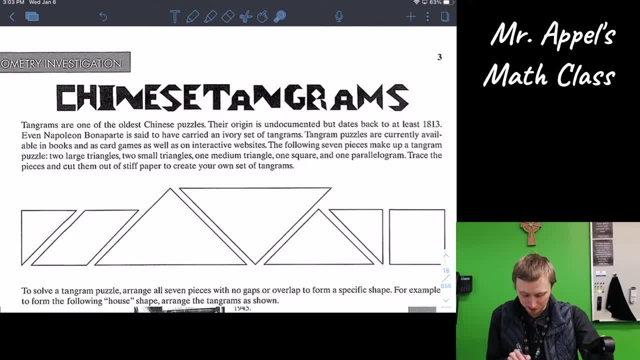 Oh, I'm sure it goes back further than that. Even Napoleon Bonaparte is said to have carried an ivory set of tangrams. Fancy. The tangram puzzles are currently available. You can find them on our website. They're available in books and as card games, as well as on interactive websites. 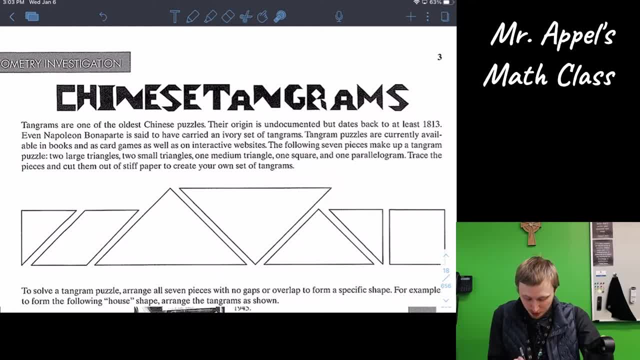 The following Seven pieces make up a tangram puzzle: Two large triangles, two small triangles, one medium triangle, one square and one parallelogram. Trace the pieces and cut them out of stiff paper to create your own set of tangrams. 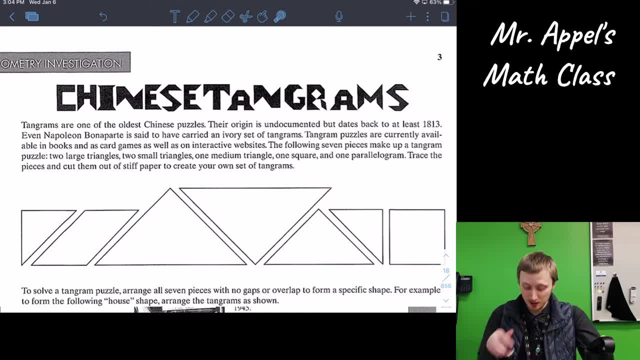 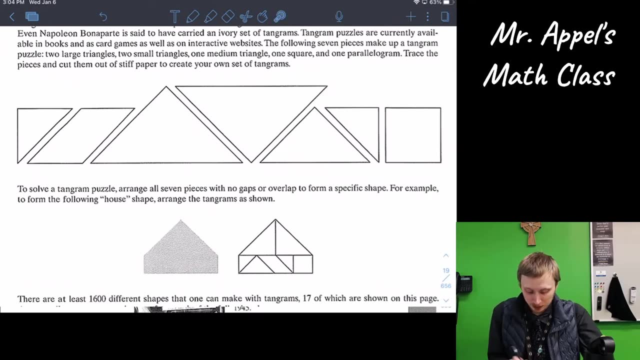 If you would like to search that up, there are sites out there with a full print-outable page You can print and then cut out the shapes. make that a little bit easier. I suggest printing it on cardstock if possible, or pick a set up from your local gaming store. 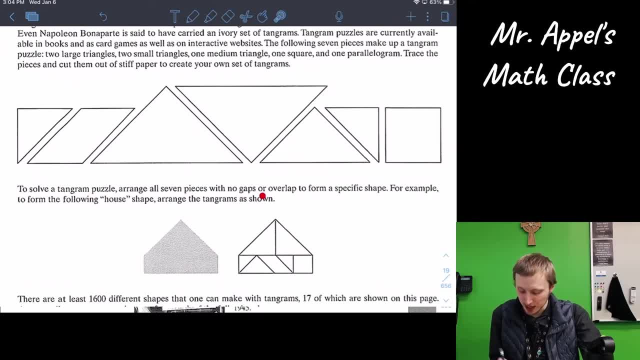 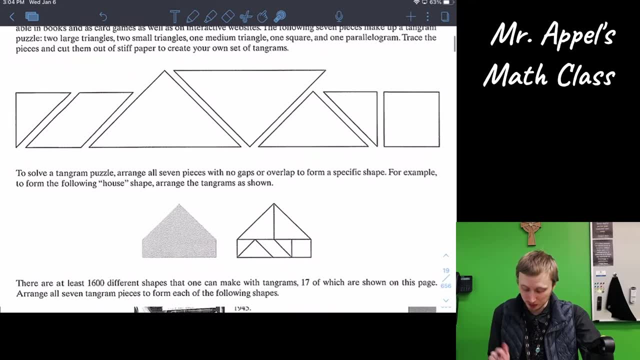 To solve a tangram puzzle, arrange all seven pieces, with no gaps or overlap, to form a specific shape, For example, to form the following house shape. arrange the tangrams as shown. So this is how the puzzle works. They give you an outline, a fully solid, shaded shape, and you need to put these pieces together. 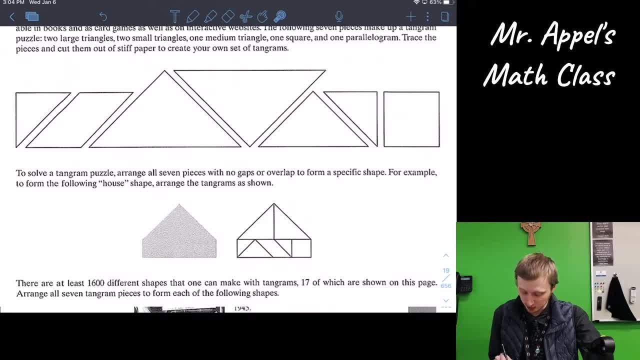 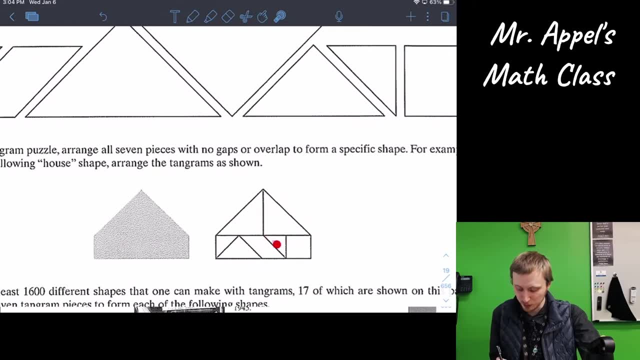 so that you create that shape. And here then is the solution showing how each of the pieces is devised. Notice the sizing there, such that the diagonal of the small triangle is the long side of the parallelogram, which is the short side of the medium triangle. 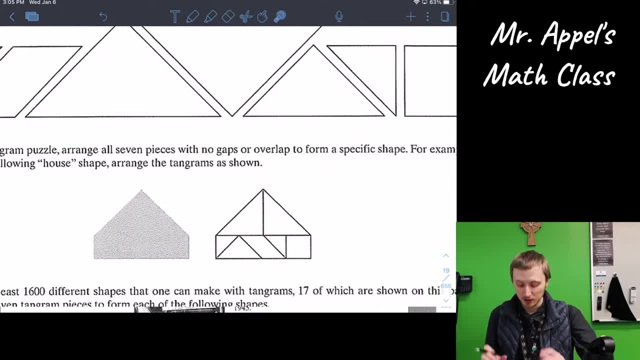 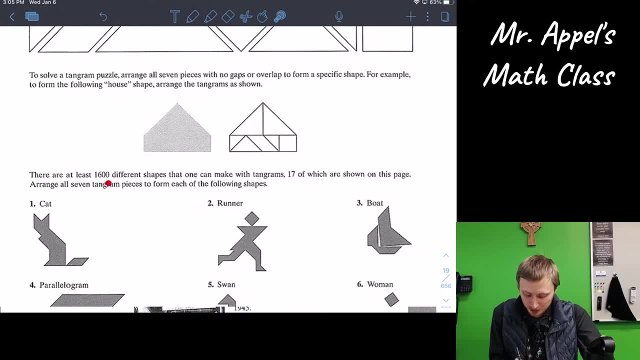 So a lot of these sizes match up to specific set of these shapes that allow you to do these things Very cool. There are at least 1,600 different shapes that one can make with tangrams, 17 of which are shown on this page. 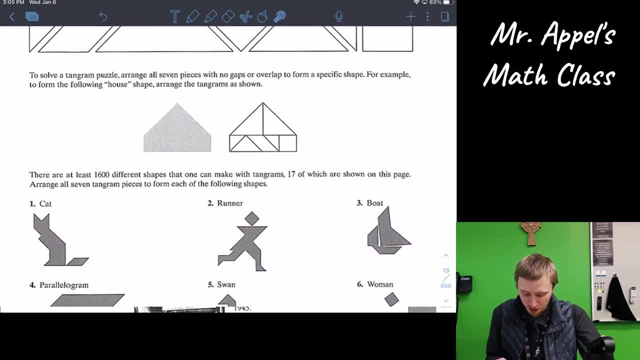 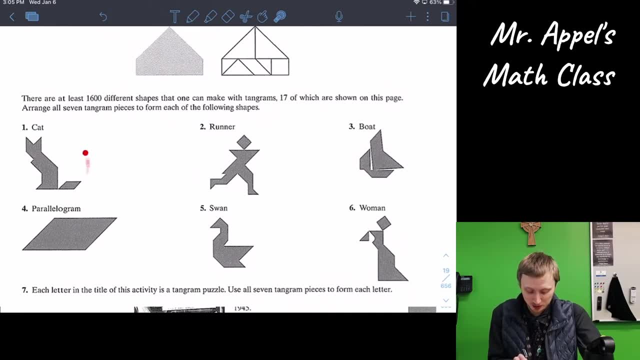 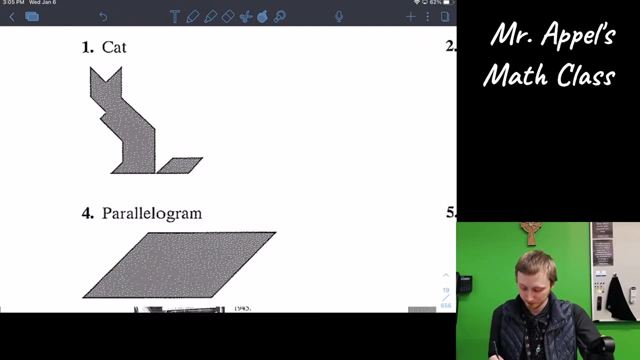 Arrange all seven tangram pieces to form each of the following shapes. So go ahead and pause there, take a screenshot, if you have a set, and try out each of these. If you would like, I will zoom in on a particular pair. 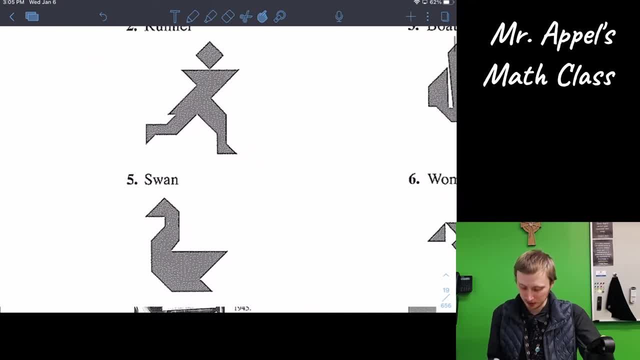 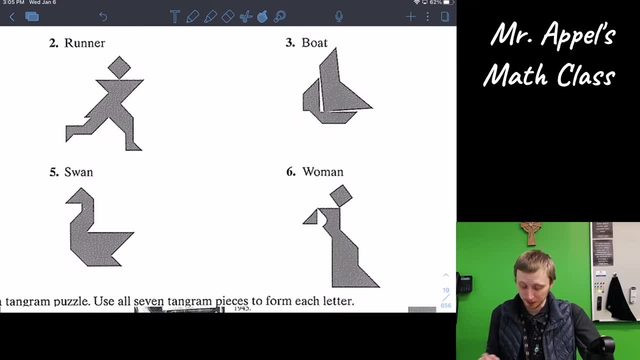 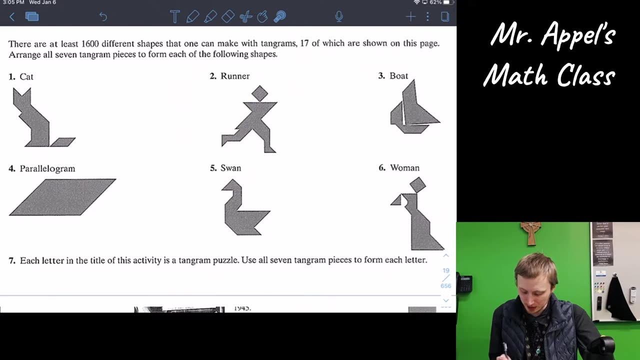 And pause it. That swan has a little extra piece on the bottom. Okay, And then the final challenge tells us: each letter in the title of the activity is itself a tangram puzzle. Use all seven tangram pieces to form each letter. 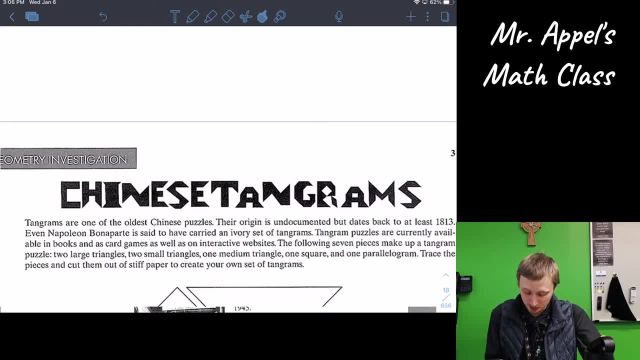 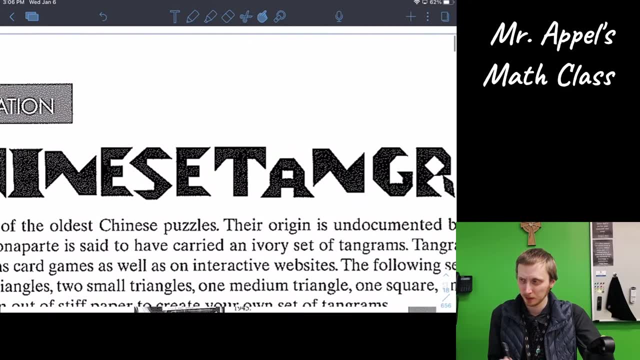 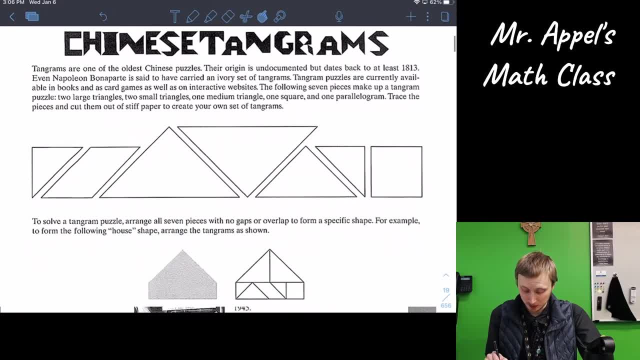 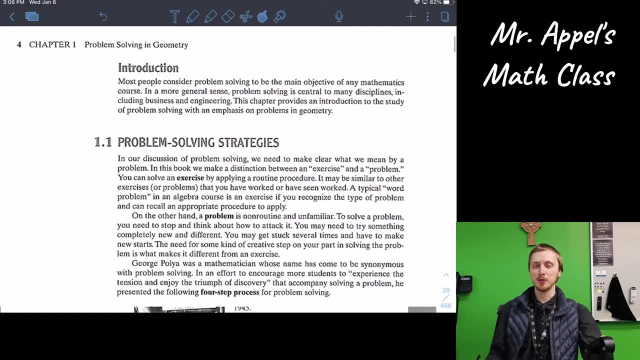 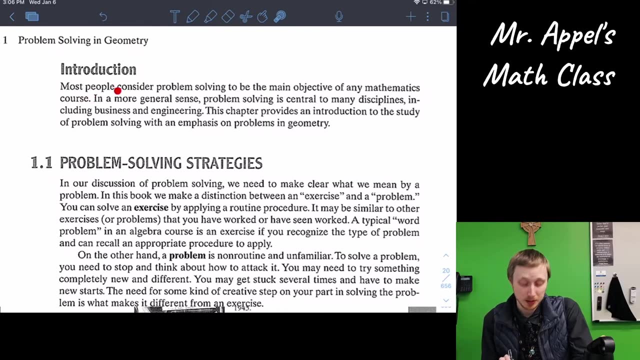 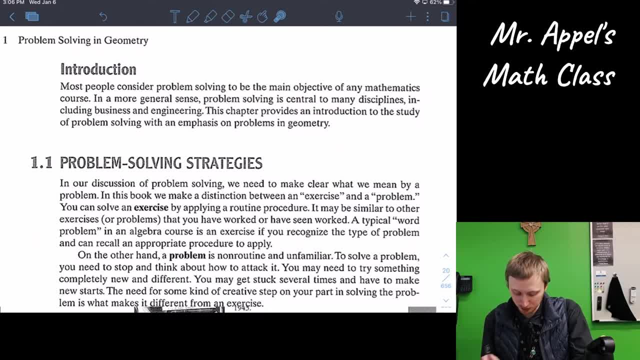 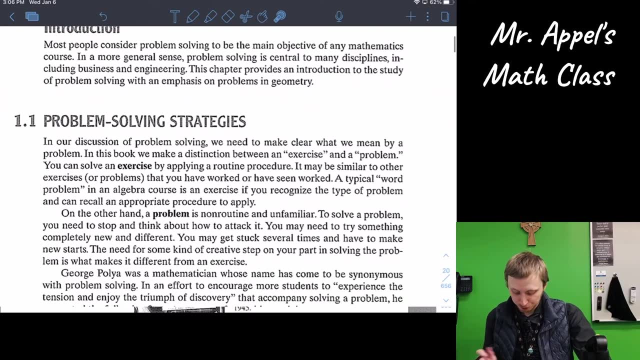 In a more general sense, problem solving is central to many disciplines, including business and engineering. This chapter provides an introduction to the study of problem solving- problem solving with an emphasis on problems in geometry- It is, after all, a geometry textbook. Section 1.1, Problem Solving Strategies. 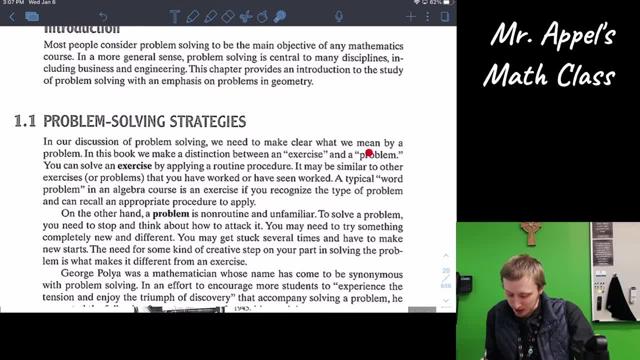 In our discussion of problem solving, we need to make clear what we mean by a problem. In this book we make a distinction between an exercise and a problem. You can solve an exercise- notice that's in bold- by applying a routine procedure. 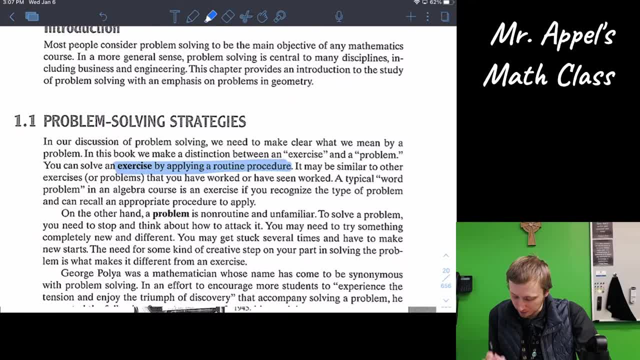 An exercise is routine. It may be similar to other exercises or problems that you have worked or have seen worked. A typical word problem in algebra course is an exercise. if you recognize the type of problem and can recall an appropriate procedure to apply, If you can read through it. 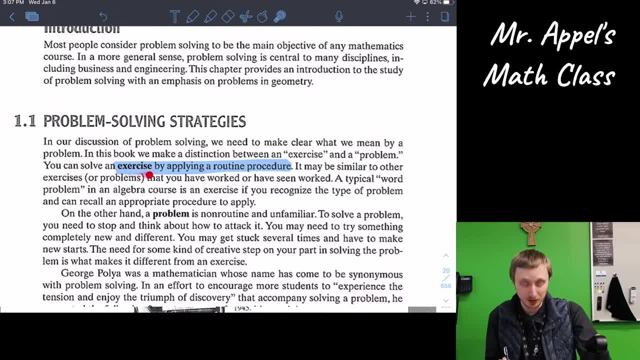 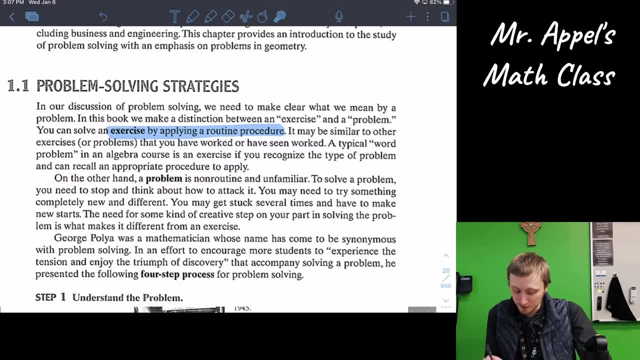 and you already know what you need to do, then it's merely an exercise. On the other hand, a problem is non-routine and unfamiliar. You read a problem and you don't know what to do right away. To solve a problem, you need to stop. 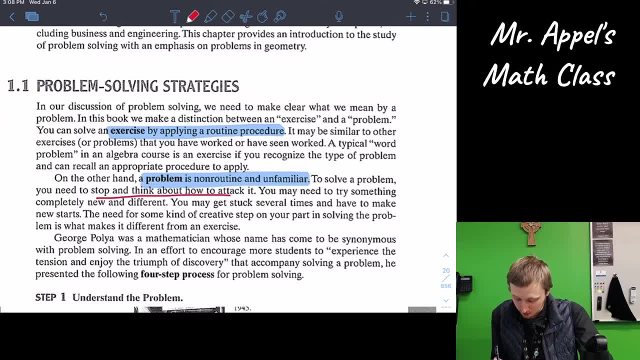 and think about how to attack it. Ooh, I like that. You may need to try something completely new and different. You may get stuck several times and have to make new starts. All right, Notice that Stuck, Restart, Restart. 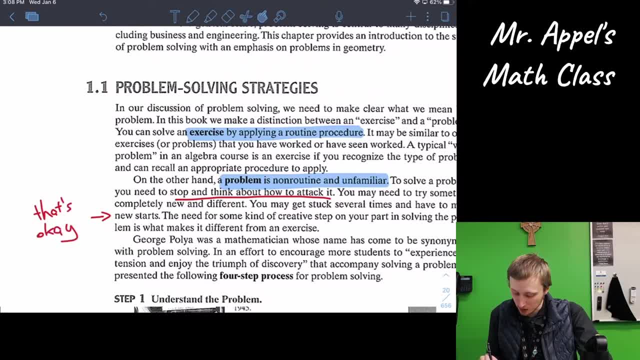 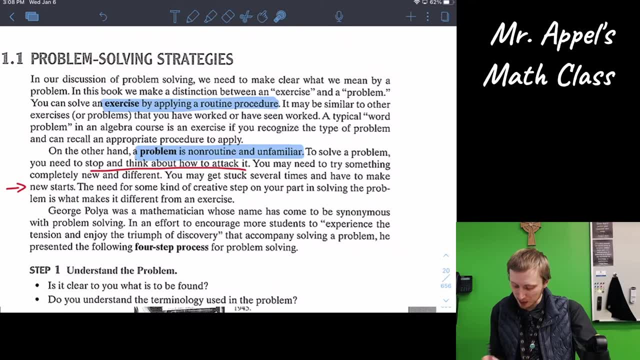 That's okay. That's part of the process. You are in fact making progress, whether you realize it or not. The need for some kind of creative step on your part in solving the problem is what makes it different from an exercise. 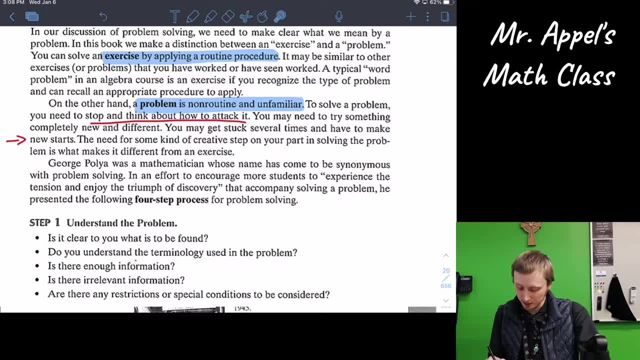 George Paglia was a mathematician. we heard him at the beginning of the section whose name has come to be synonymous with problem solving, In an effort to encourage more students to experience the tension and joy, the triumph of discovery, that accompany solving a problem. 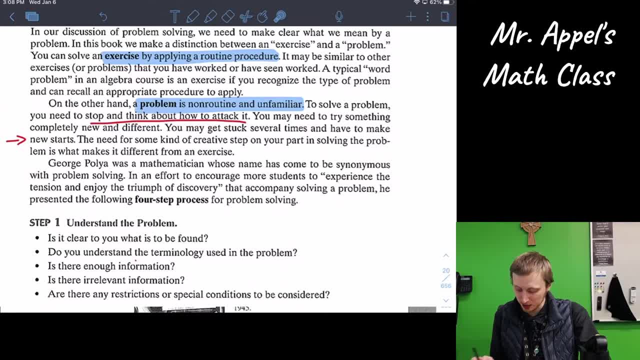 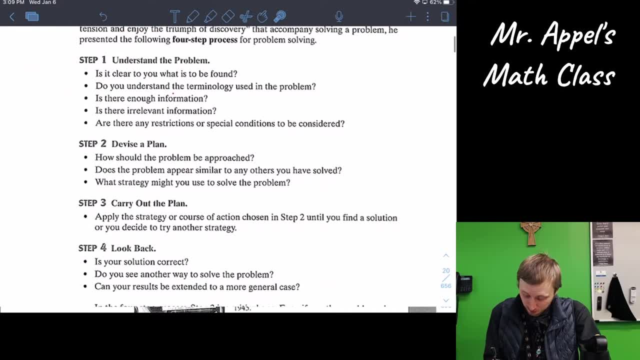 he presented the following four-step process for problem solving. So this is going to be huge right. This will form the foundation of this entire section. In fact, this, both sections, this whole chapter will be built around utilizing these four steps. 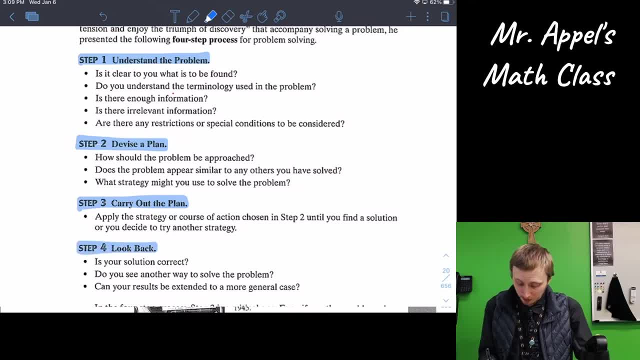 So we better know them well. Step one: understand the problem. Of course you need to read through it and then make sure: do you actually understand what it's saying? What is the problem asking? Is it clear? you know what to be found. 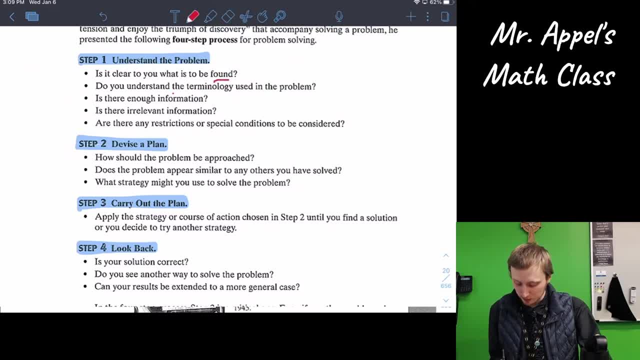 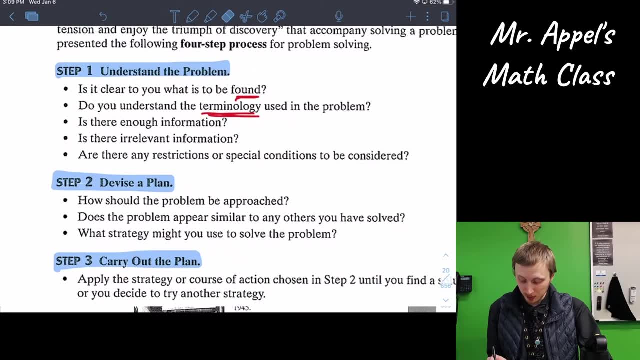 Do you understand the terminology? Okay, What are you looking for? Vocabulary, right. Are there any words? Are there any words that you don't know? that might be confusing you and thus confusing the whole problem? Is there enough information? Is there irrelevant information? 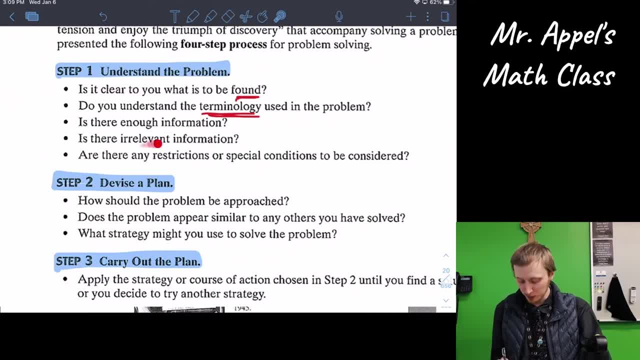 Good old algebra word problems. try to trip you up with throwing in extra stuff you don't need. Are there any restrictions or special conditions to be considered? Oh, this is a good one, right, Always think about. I don't need it in quotes, but 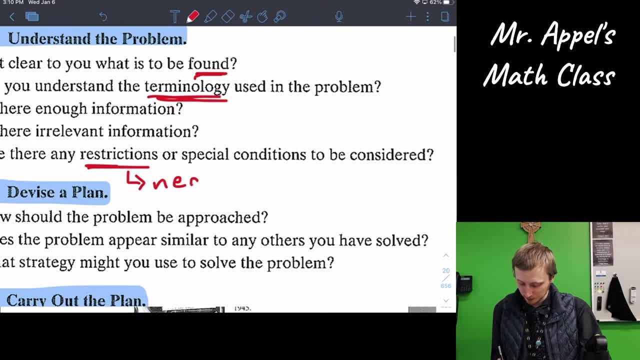 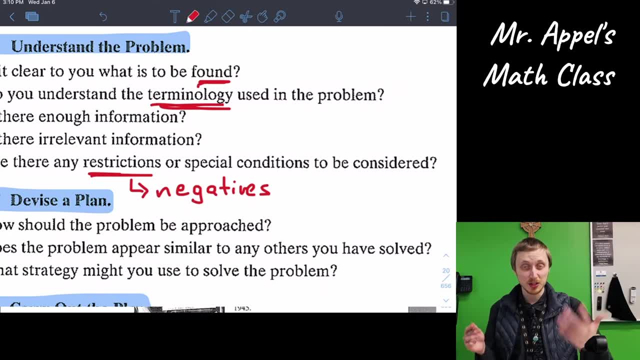 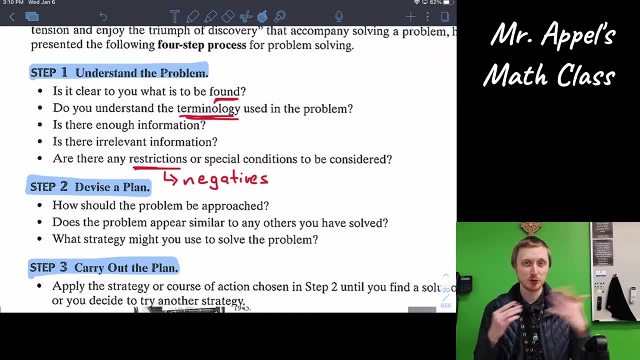 oops, Come on, let me write. Negatives is a good case to consider, especially with real world problems. Very often things in life cannot have measurements and lengths and distances and time and money. You will not have negative values for. 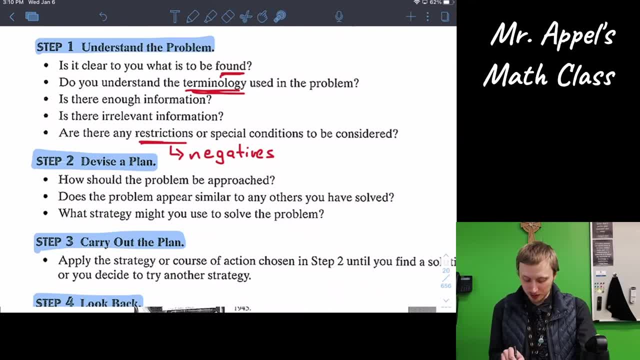 So, after you understand what's all going on, next step: devise a piece of paper Plan. Start putting together an attack strategy. How should the problem be approached? Does the problem appear similar to any others you have solved? Does it remind you of anything? 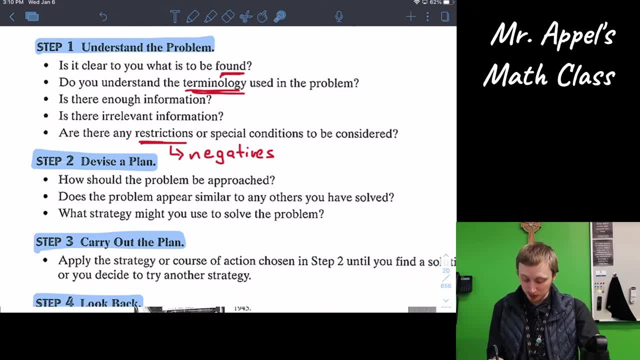 What strategy might you use to solve the problem? And that sometimes can answer the question of how? How can you solve it? Use one of the strategies right. We will have six of them in this chapter: three in the first section and three in the latter section. 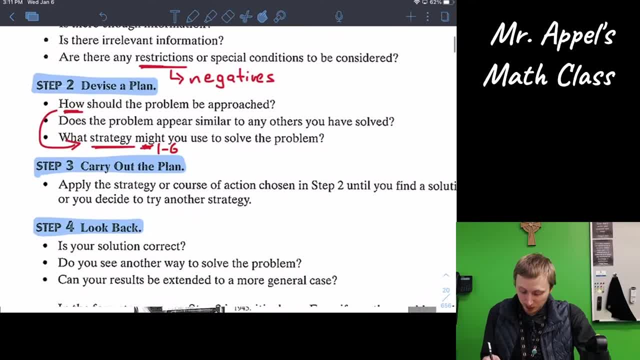 Next video. Step three: Carry out the plan. Once you have a plan, of course, it only is useful to you if you make use of it. So apply that strategy or course of action that you chose in step two until you find a solution. 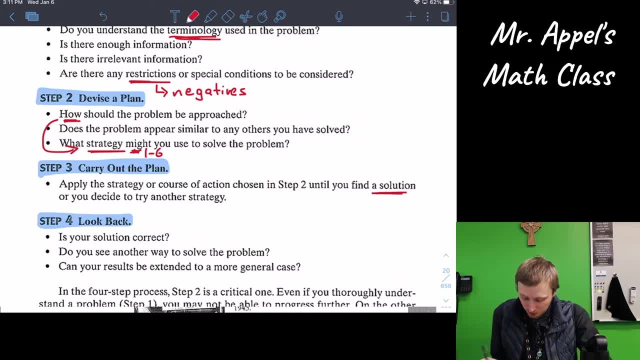 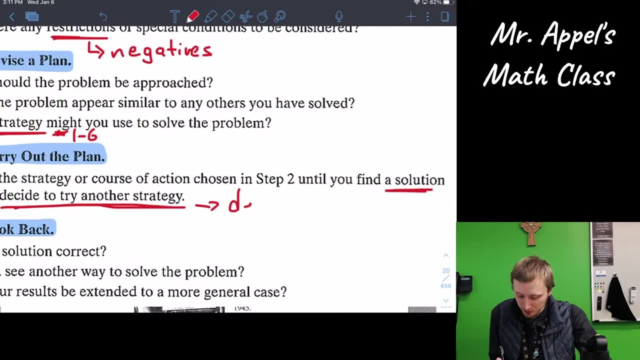 or a solution, or decide to try another strategy- Right, Because it's very possible you'll run into a dead end right and have to restart, or you might just learn something new that will clue you in as to a better strategy. 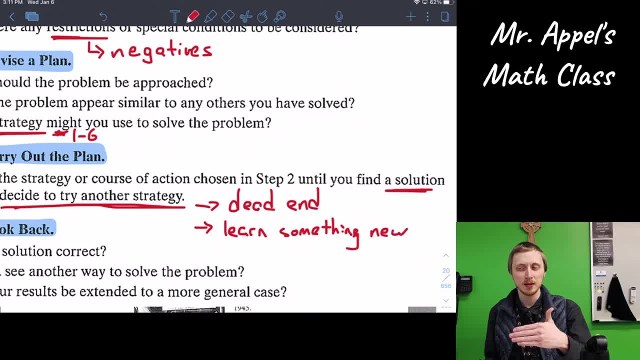 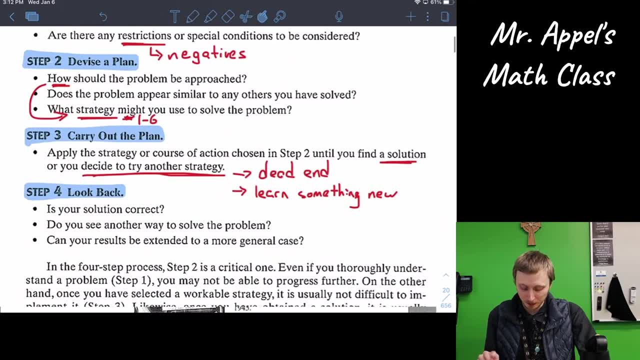 and you realize: ooh, wait, now I see something I didn't before. Let me go back, try a different one that I think will get me there faster or more efficiently. And then step four, especially after you run into a dead end. 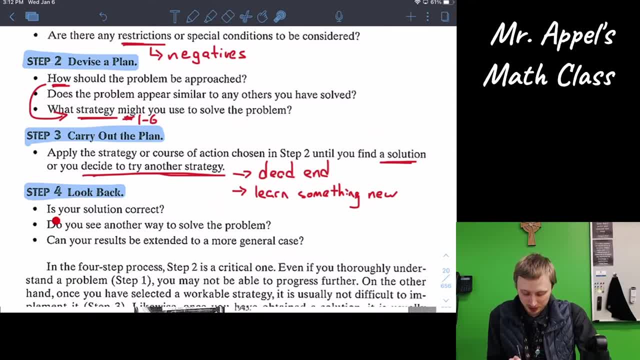 or run into one of these. look back: Is your solution correct? Check your work right. Do you see another way to solve your problem, especially once you learn something new, even if you already have it correct? Ask yourself: was that the only way? 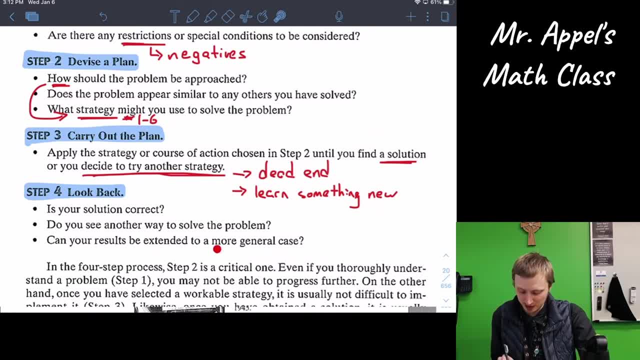 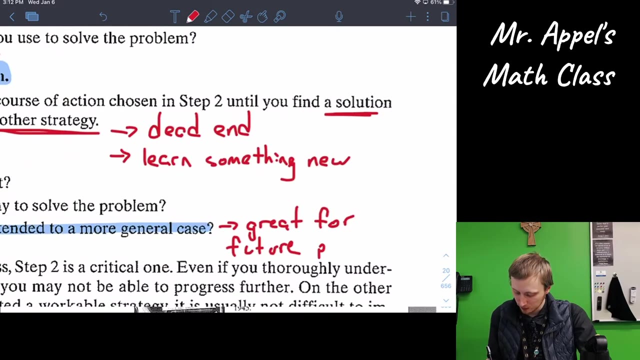 Could there have been another solution out there? Can your results be extended to a more general case? This is really handy. Okay, Step four: future problems. So if you want to not just solve this but set yourself up for success in the future, 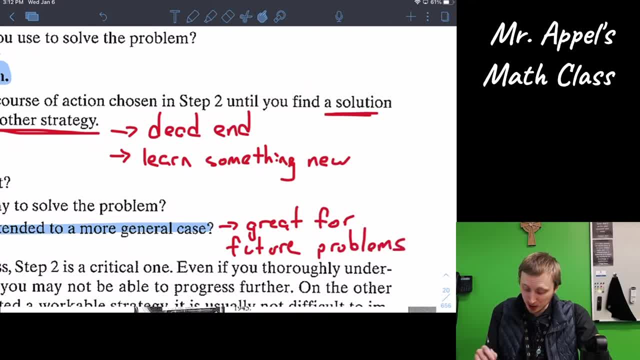 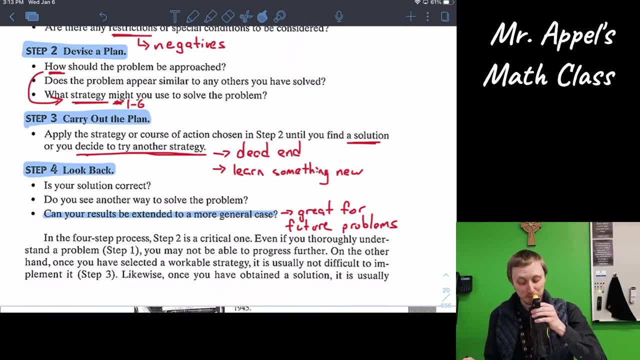 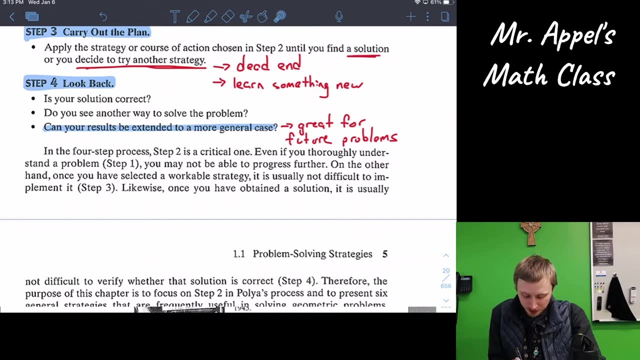 really stop and consider how can I generalize this problem so that I could use it as a template when next I encounter a similar problem In the four-step process? step two is a critical one, Even if you thoroughly understand a problem. step one. 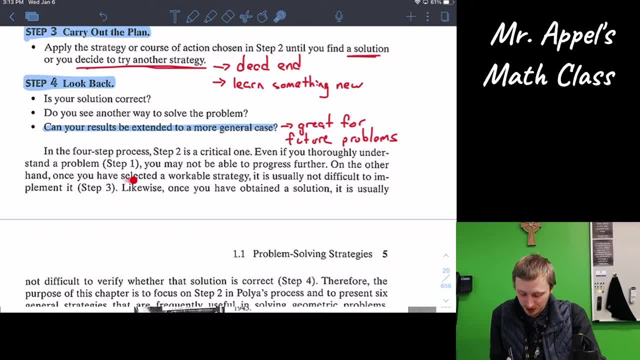 you may not be able to progress further. On the other hand, once you have selected a workable strategy, it is usually not difficult to implement Step three right. It's the picking out of the strategy that is the real thinking part. 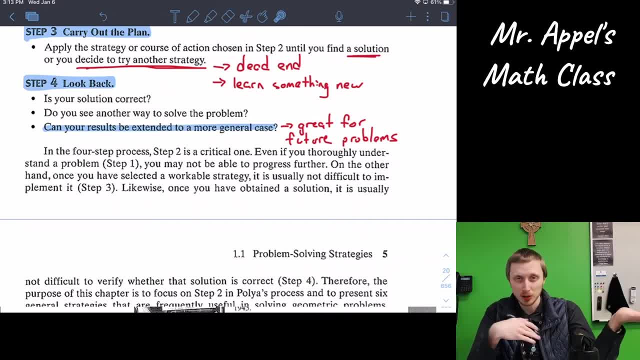 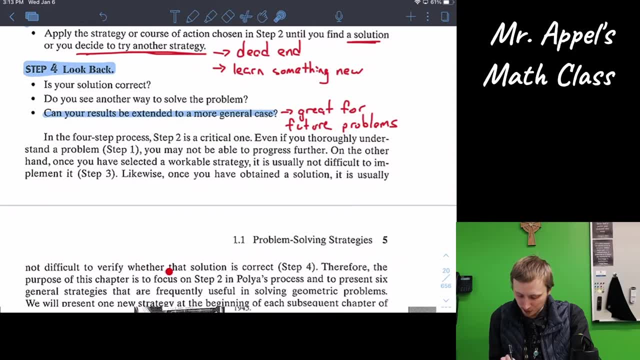 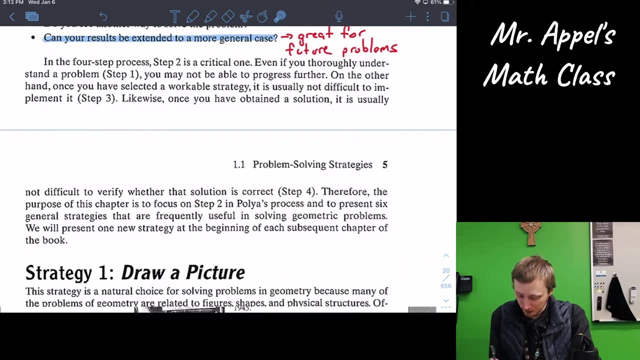 Carry out the plan is literally procedural. You could. The computer could do that part. Likewise. once you have obtained a solution, it is usually not difficult to verify whether that solution is correct. Therefore, the purpose of this chapter is to focus on step two in Pauli's process. 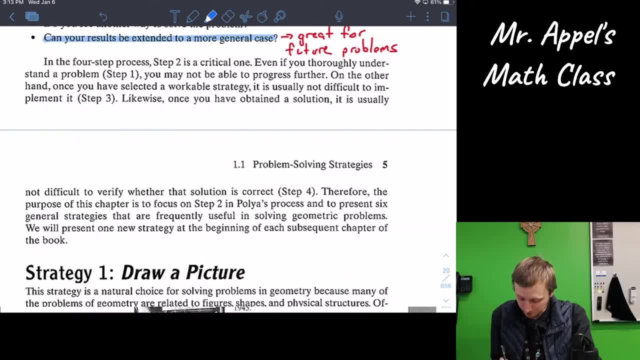 and to present six general strategies that are frequently useful in solving geometric problems. We will present one new strategy at the beginning of each subsequent chapter of the book, as said before. So with that, set up that four-step process in the back of our minds. 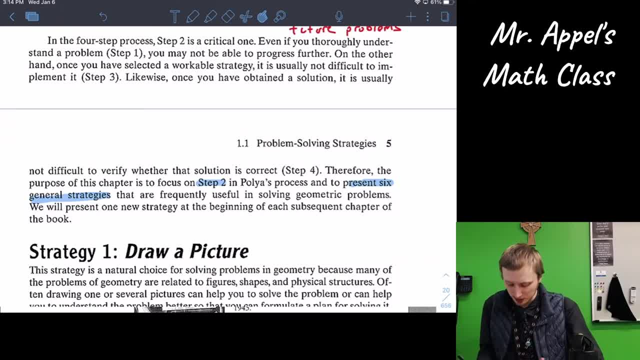 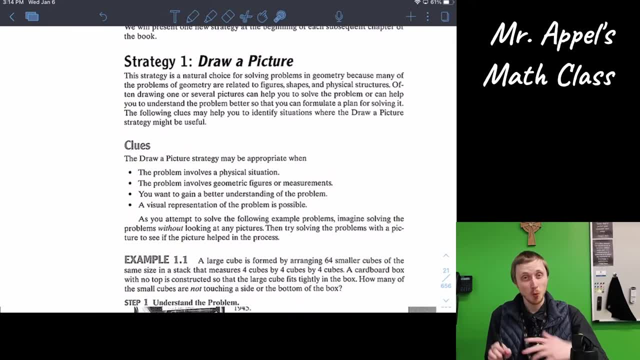 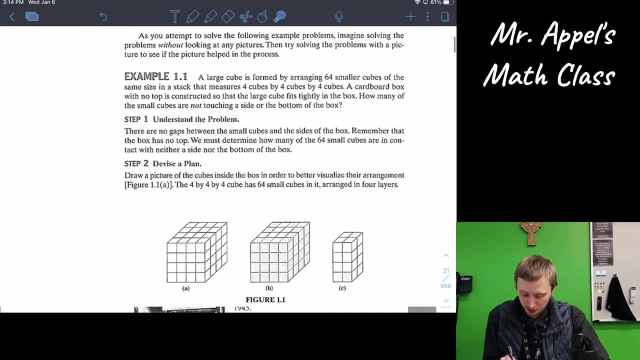 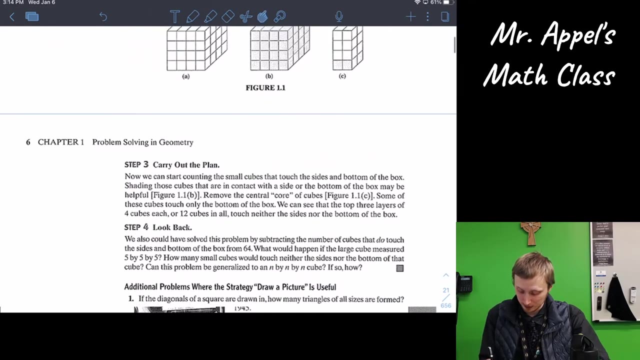 let's work through these three new strategies. that will all include a short description, some clues as to when they might be the best strategy to use and an example complete with the full one, two, three and four steps, And then, at the end of each one, 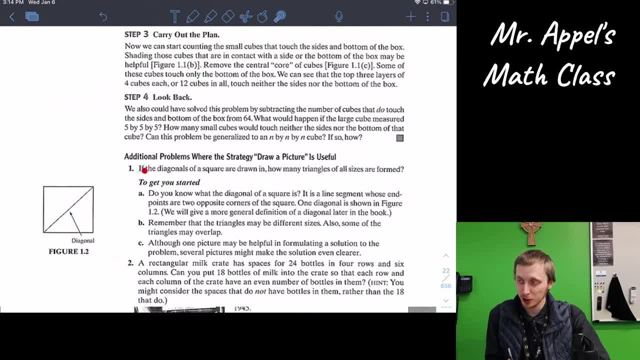 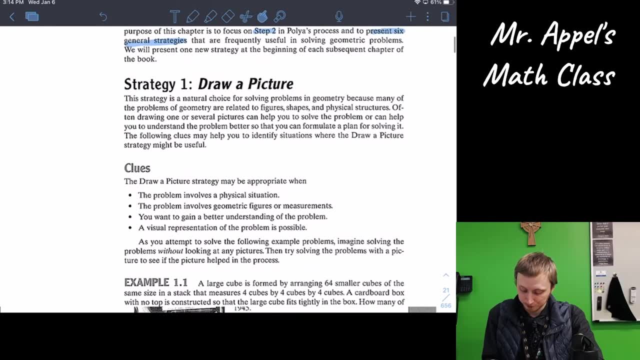 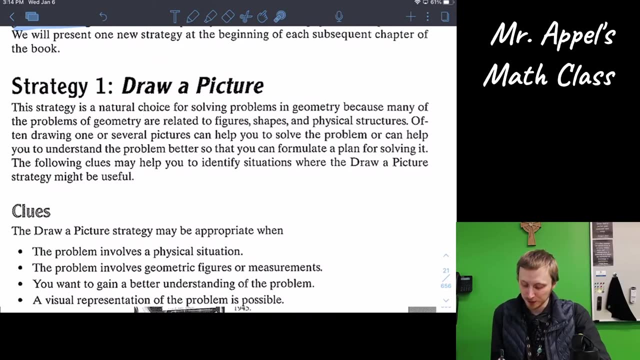 a pair of additional problems for you to practice on your own. Let's go. Let's go through each of those in turn. Strategy number one: Draw a picture. This strategy is a natural choice for solving problems in geometry, because many of the problems of geometry 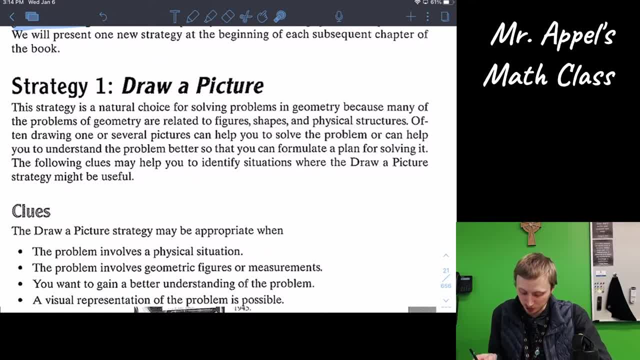 are related to figures, shapes, physical structures. Okay, That's some good stuff. Often, drawing one or several pictures can help you solve the problem, or can help you understand the problem better so you can formulate a plan for solving it. Wait, 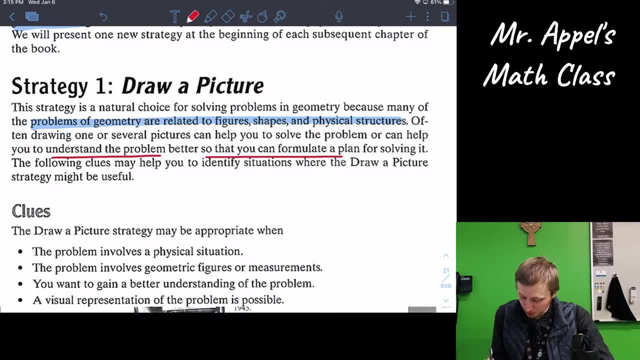 Understand so you can formulate a plan for solving it. That's saying that this strategy will help lead you to picking out another strategy. Okay, So keep that in mind that this by itself does not solve the problem. The following clues may help you identify situations. 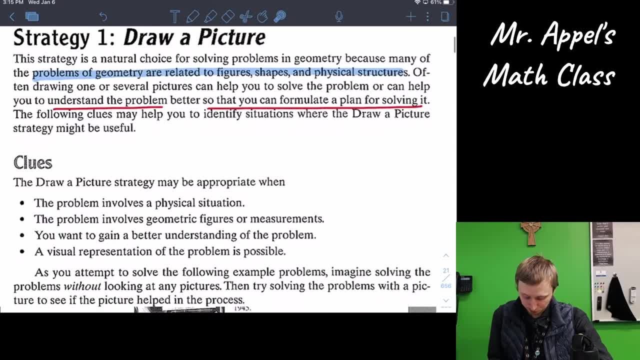 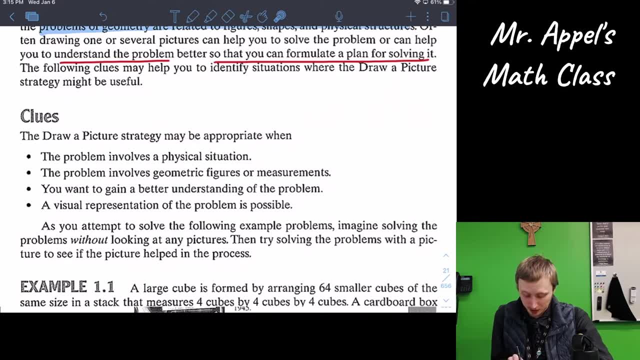 where the draw a picture strategy might be useful. So, anytime the problem involves a physical situation, draw a picture might be appropriate. Anytime the problem involves geometric figures or measurements- physical situation figures, measurements- you want to gain a better understanding of the problem. 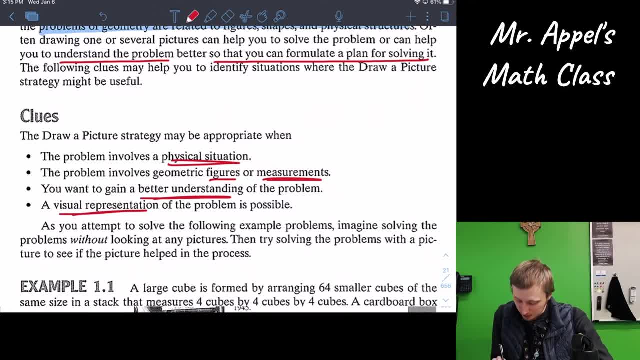 A visual representation is possible right, Or even already presented right. One thing they don't note here is what if the problem itself already gives you a picture, you might want to draw another picture. That's entirely possible too, As you attempt to solve the following example problems. 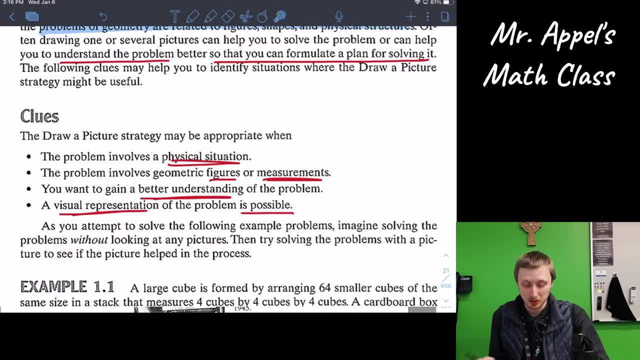 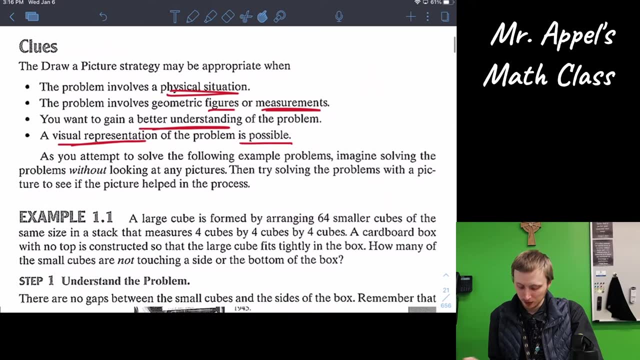 imagine solving the problem without looking at any pictures To contrast how hard it would be. Then try solving the problems with a picture to see if the picture helped in the process. So here we go. A large cube. Example one: A large cube is formed by arranging 64 smaller cubes. 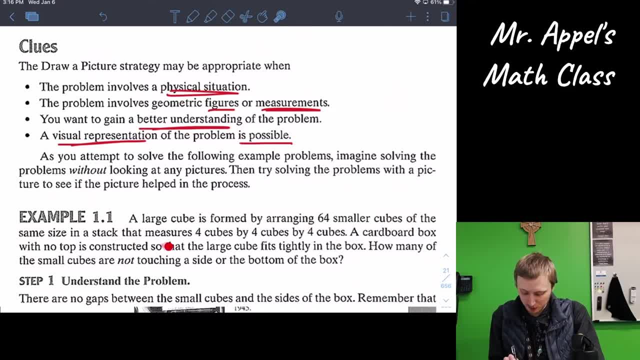 of the same size. in a stack that measures four cubes by four cubes, by four cubes, A cardboard box with no top is constructed so that the large cube, that one made of 64 small ones, fits tightly in the box. How many of the small cubes are not touching a side? 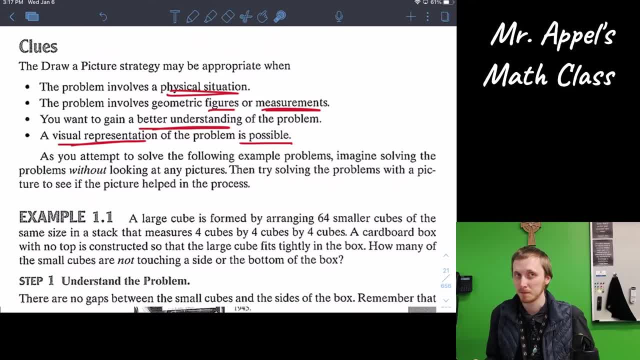 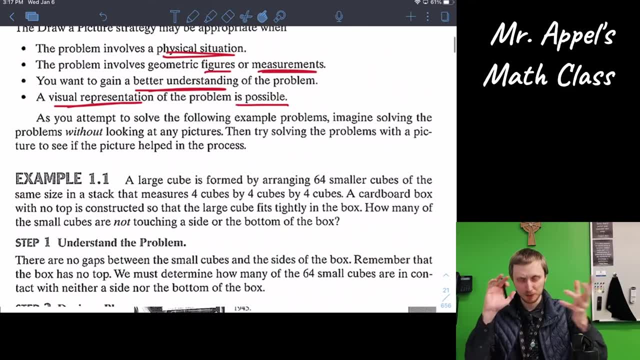 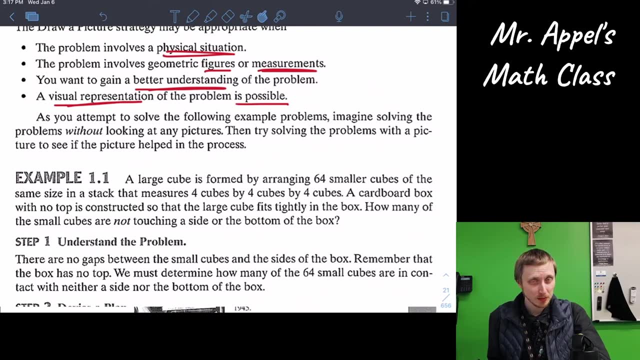 or the bottom of the box. Okay, You got all that in your head. How is your spatial reasoning? Go ahead and pause the video here. Give that problem a consideration. Maybe give it an attempt if you're feeling ambitious, And then come back for the solution. 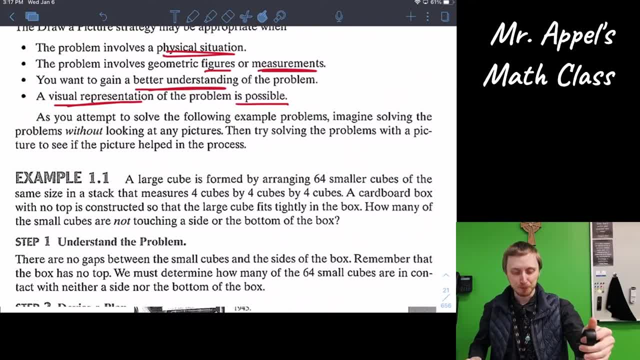 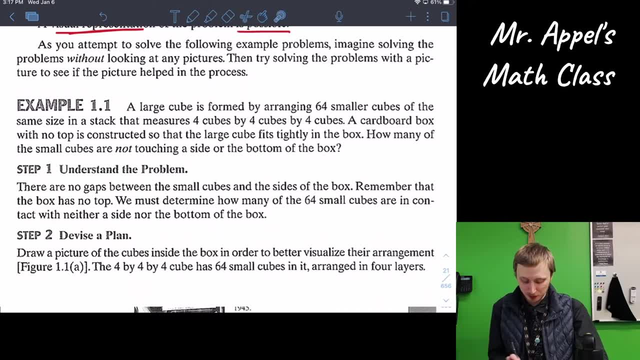 Welcome back. All right, Here we go. Step one: You need to understand the problem. What is going on? What is it asking for? Notice: there are no gaps between the small cubes and the sides of the box. Remember, it fits tightly. 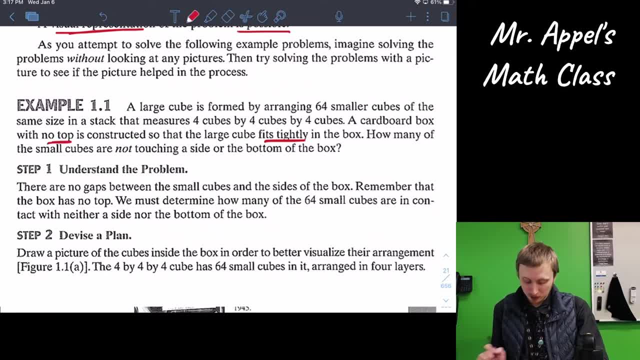 Remember that the box has no top. I said that Okay, So a box normally has six total faces. Take away the top, You're left with five. Now let's determine how many of the 64 small cubes are in contact with neither a side nor the bottom. 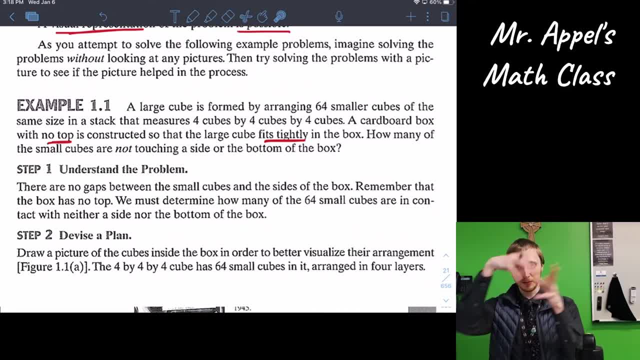 Okay. So, thinking about that, it seems like they should be somewhere, you know, in the middle-ish. That's our understanding, But how many of them are there? That's what we want to know. So we're going to devise a plan. 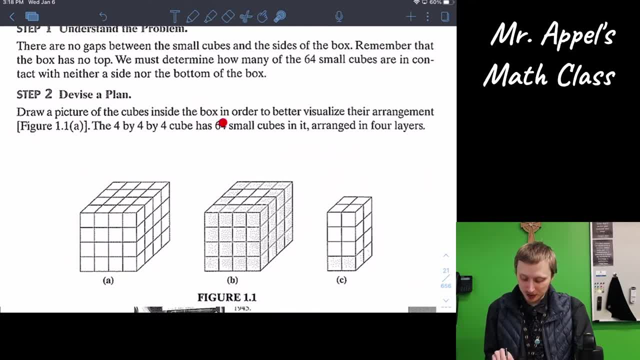 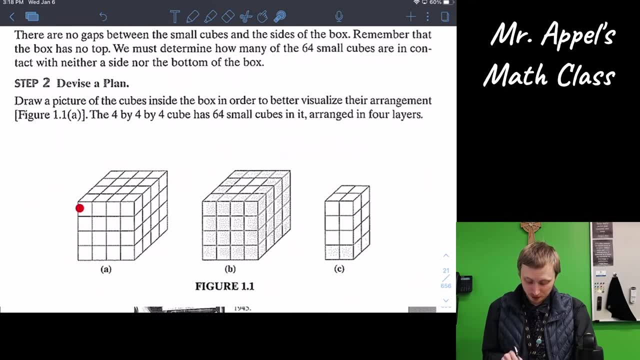 Our plan is to draw a picture of the cubes inside the box in order to better visualize their arrangement. So we're going to start with the 411A. So here we have the 4 by 4 by 4, cube 64 total, because 4 times 4 times 4 is 64.. 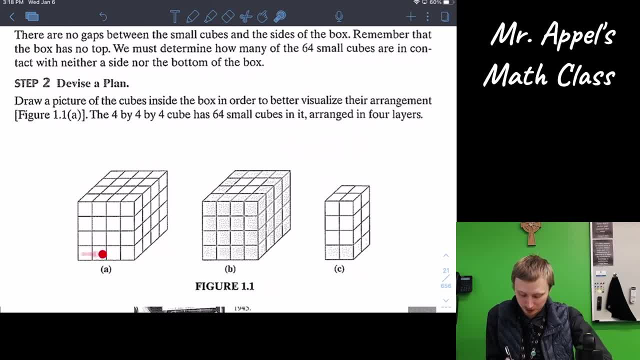 And it is arranged in those four layers. If you think about this layer here and we could you know invisibly behind there you have that back layer of cubes here And stack four of those on top of each other to get all 64.. 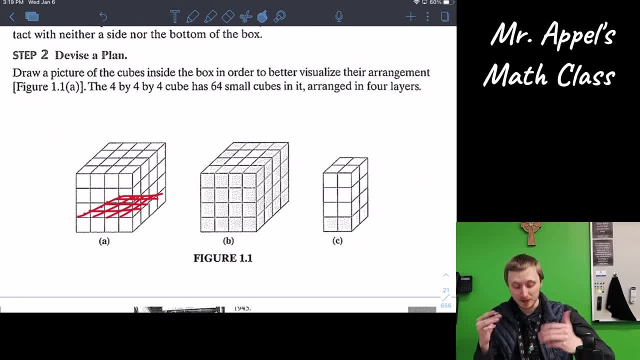 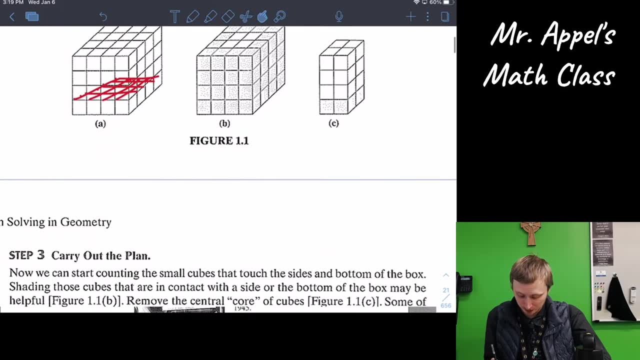 Now we're going to start carrying out our plan. Now that we have our picture, let's build upon our picture in order to count down how many cubes are left. That's step three: carrying out the plan. Now let's see if I can get. 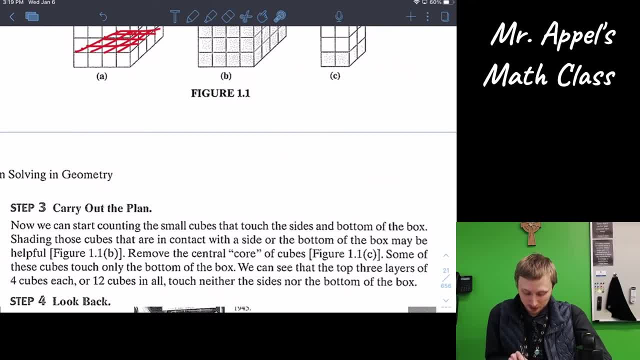 not quite everything on screen, unfortunately. Now we can start counting the small cubes that touch the sides and bottom of the box. Those will be the cubes that will just be the sides and bottoms of our entire cube Shading, those cubes that are in contact. 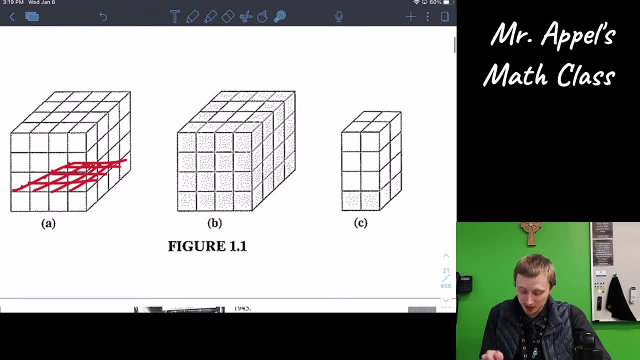 with a side of the bottom of the box may be helpful. Okay, it's a little hard to see in this copy, but they have gone ahead and shaded this entire face And this entire face And then, because this face is attached to this top face of that cube- 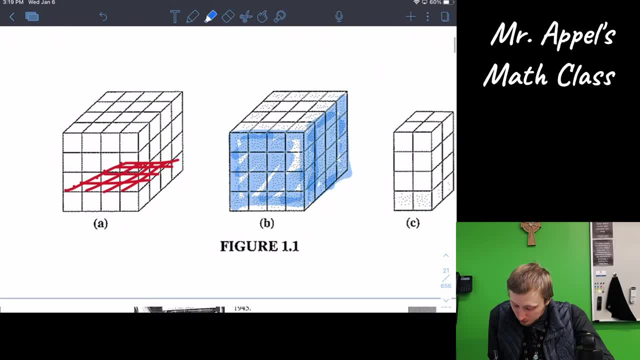 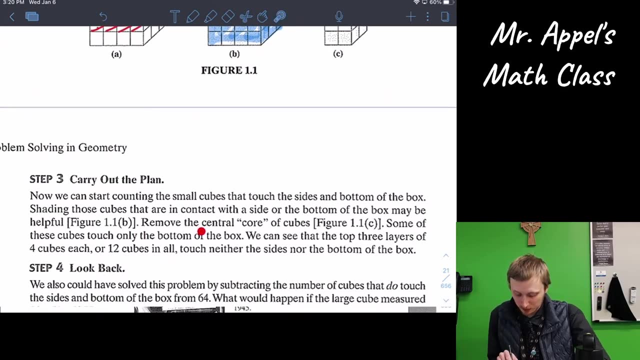 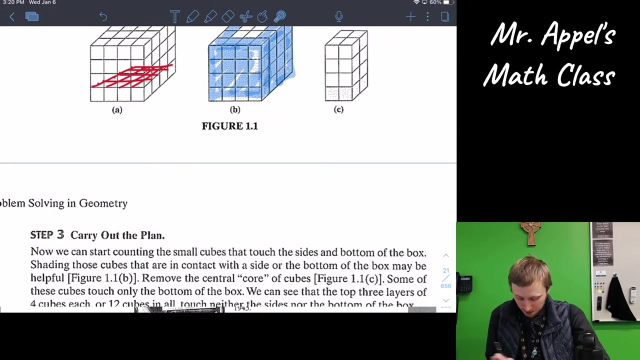 we also shade this region right here, not touching those center four. Okay, Remove the central core of cubes seen here in figure C. Some of those cubes touch only the bottom of the box. That would be these guys down here. We can see that the top three layers. 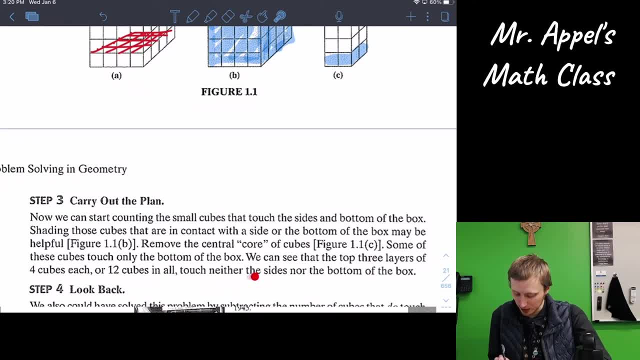 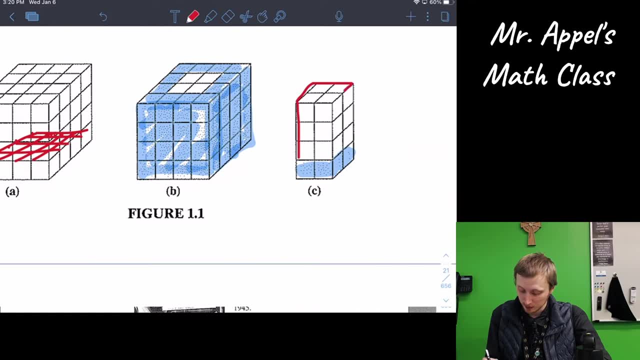 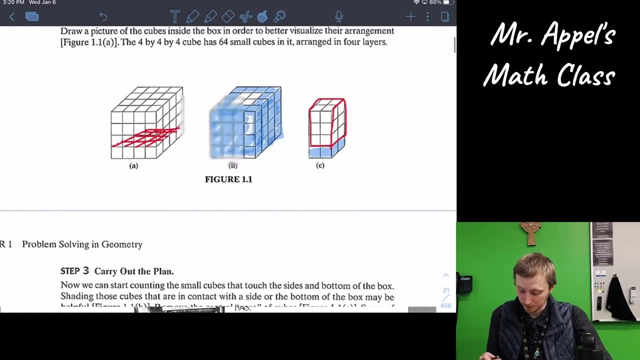 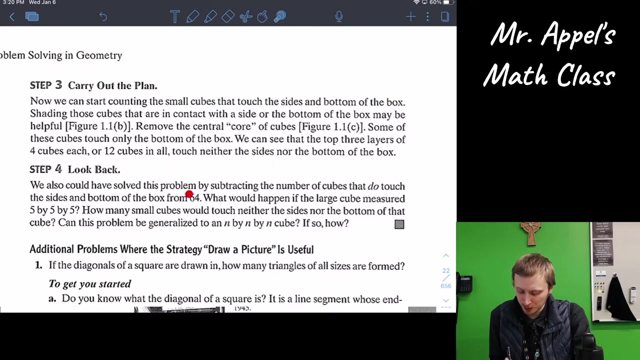 of four cubes each, or 12 cubes in all, touch neither the sides nor the bottom of the box. That would be right, this little prism of what is left. So step four: looking back, We could also have solved this problem. 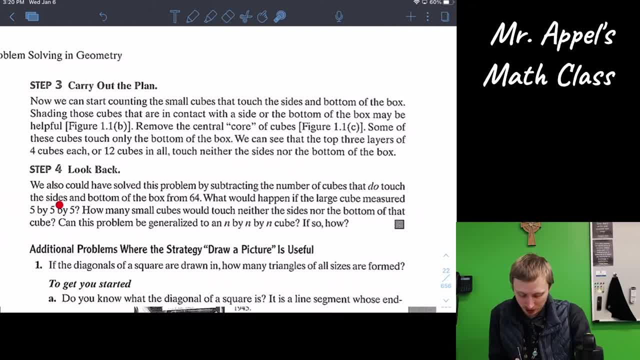 by subtracting the number of cubes that do touch the sides and bottom of the box from 64. So you could think of it as a mathematical count instead of just a visual elimination. What would happen if the large cube measured five by five, by five? 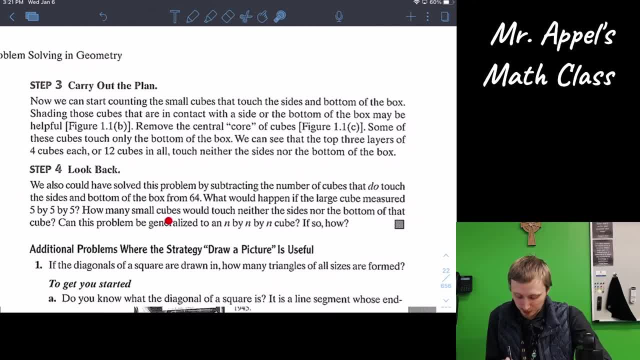 This is our generalization. What if it was a bigger problem? How many small cubes would touch neither the sides nor bottom of that cube? Can this problem be generalized to n by n by n? If so, how Right Could you go? bigger and bigger and bigger. 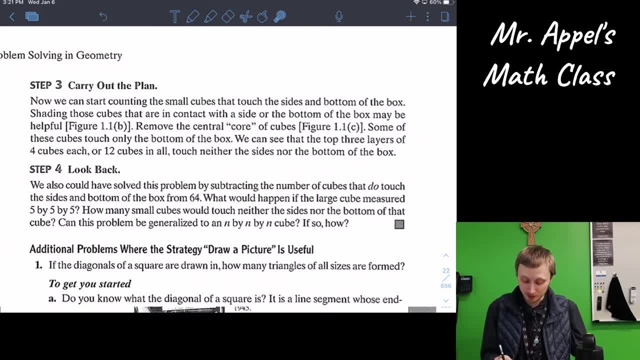 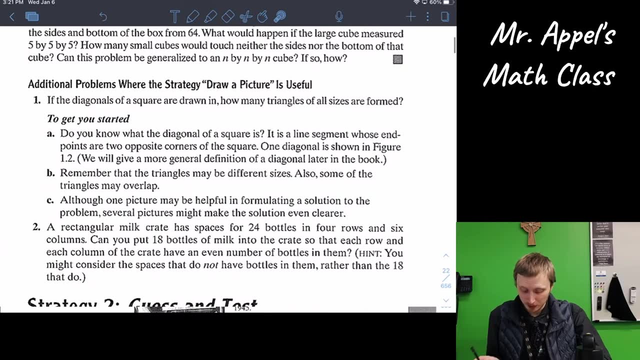 And what's the general case? All right again, this is future-proofing your understanding of this problem, making it the most useful to you. All right, if you want to try practicing that yourself. here are some additional problems We have. first off. 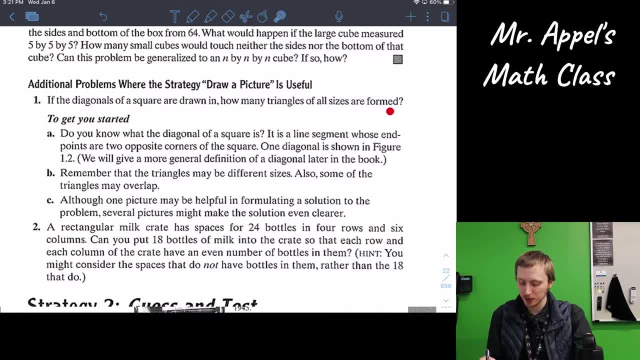 if the diagonals of a square are drawn in, how many triangles of all sizes are formed. And they've even given you some tips. First off, do you know what the diagonal of a square is? It's part of that understanding. There's a line segment whose end points 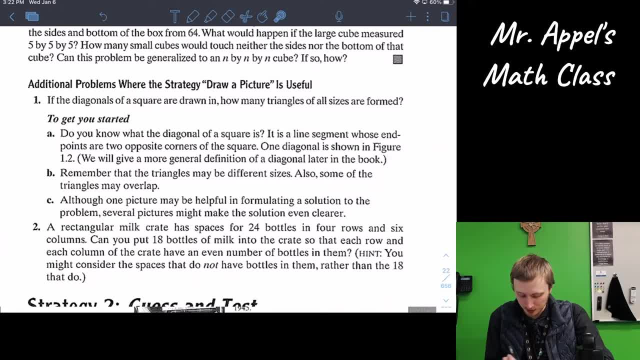 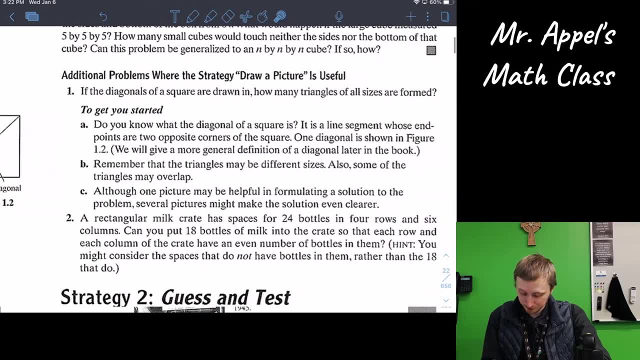 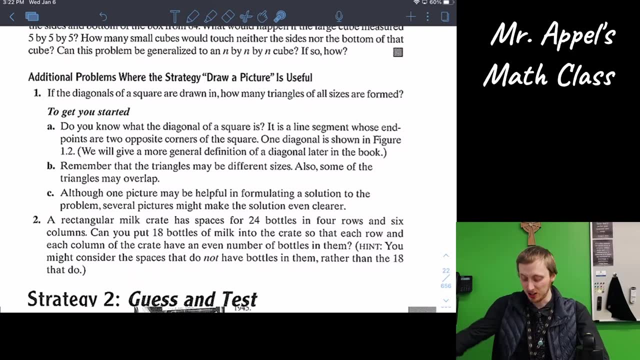 are two opposite corners of the square. One diagonal is shown in figure 1.2.. This is the diagonal. It is one of the diagonals. We will give a more general definition of a diagonal later in the book when you get to the more geometric stuff and definitions. 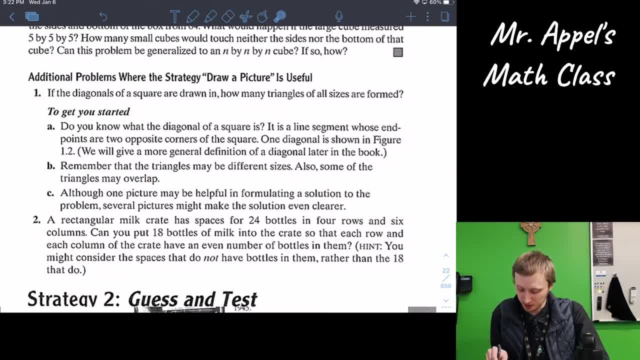 Remember that the triangle may be different sizes. Also, some of the triangles may overlap Right All possible triangles. Although one picture may be helpful in formulating a solution to the problem, several pictures might make the solution even clearer. Hmm, It's a relatively simple diagram. 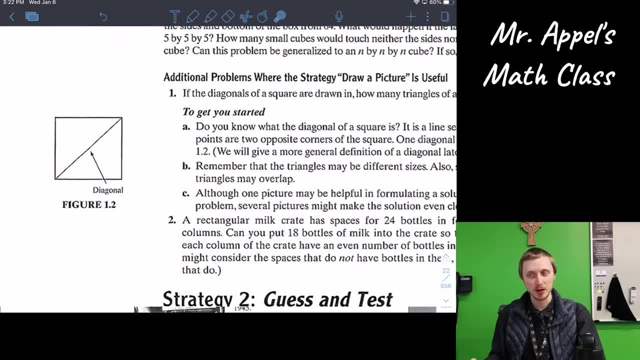 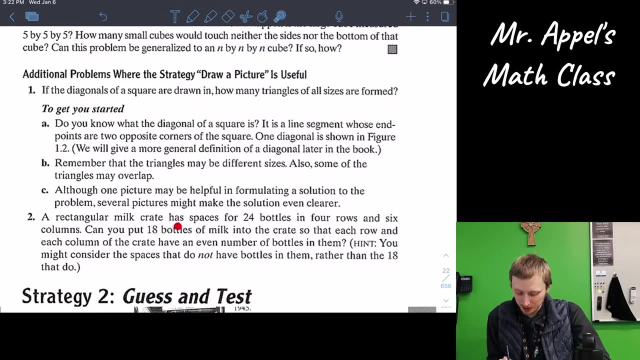 but don't let this fool you into thinking this is all that there is. Maybe to keep track of the triangles, you want to draw different renditions of the different sizes And then second draw a picture. problem: A rectangular milk crate has spaces for 24 bottles. 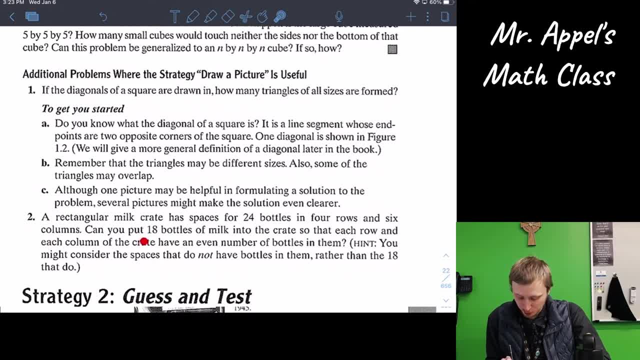 in four rows and six columns. Can you put 18 bottles of milk into the crate so that each row and each column of the crate have an even number of bottles in them? you might consider the spaces that do not have bottles in them, rather than the 18 that do. 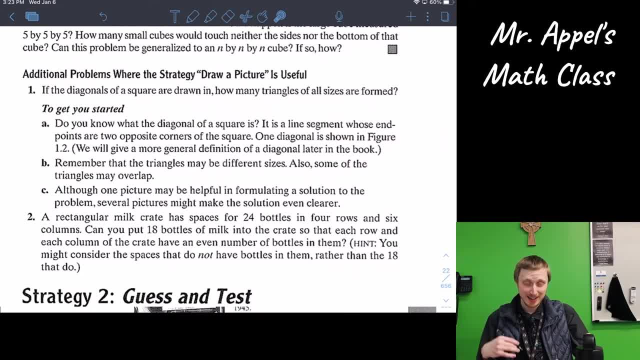 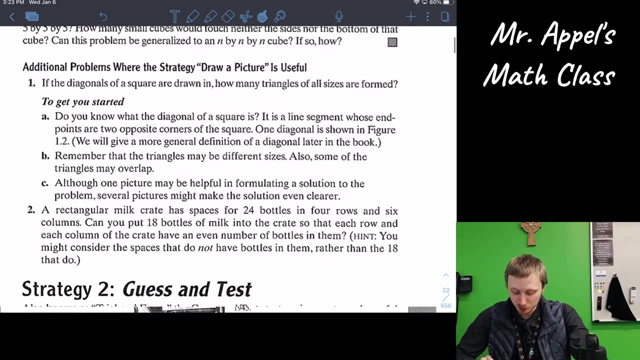 This being, of course, 24 minus 18, leaves you with only six items to arrange and consider, instead of all 18.. All right, now that you've had a chance to try those problems, let's look at strategy number two: Guess and test. 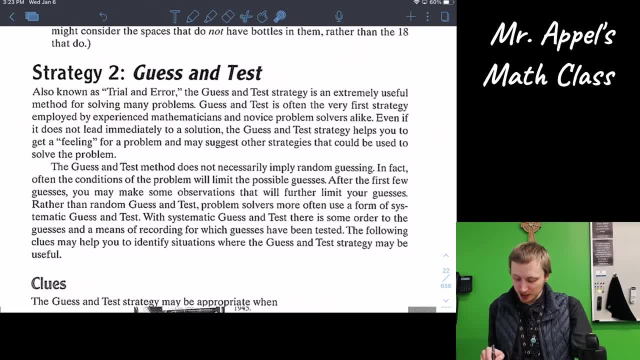 Also known as trial and error. the guess and test strategy is an extremely useful method for solving many problems. A lot of people use it all the way down into elementary school and it's still good up into high school adulthood. Guess and test is often the very first strategy. 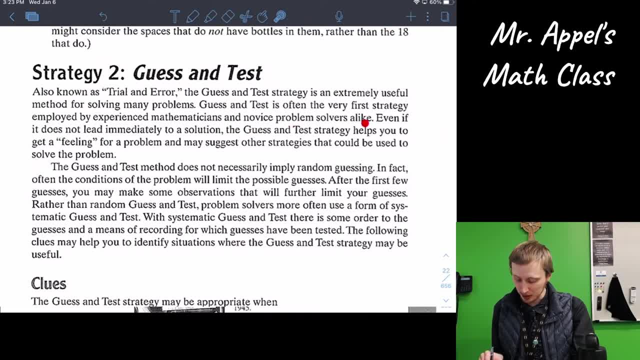 explored by experienced mathematicians and novice problem solvers alike. Hey, that's what I said. Even if it does not lead immediately to a solution, the guess and test strategy helps you to get a feeling for a problem and may suggest other strategies that could be useful to solve the problem further. 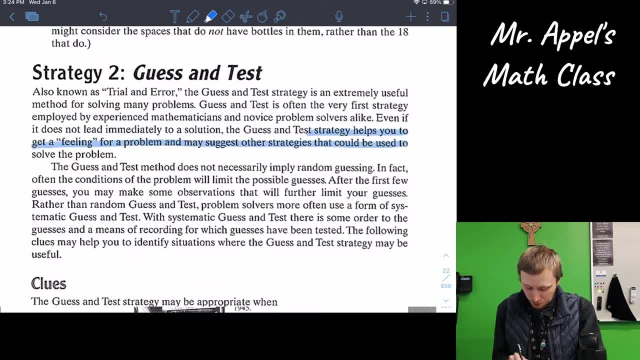 I'll go ahead and highlight that one as well. So, similar to the drawing a picture, this might not get you the actual answer right away, but it will set you up to make the next strategy that much more potent and easier. The guess and test method. 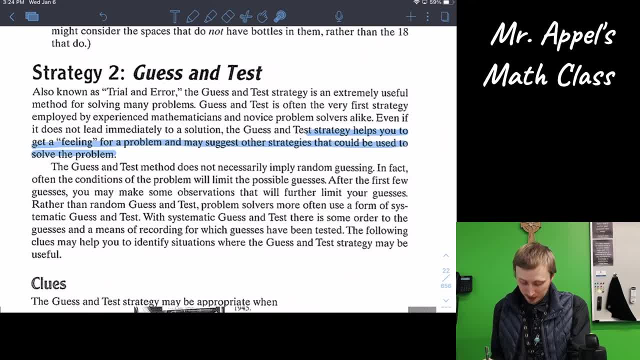 does not necessarily imply random guessing. In fact, often the conditions of the problem will limit the possible guesses. After the first few guesses you may make some observations that will further limit your future guesses. Rather than random guess and test, problem solvers more often use 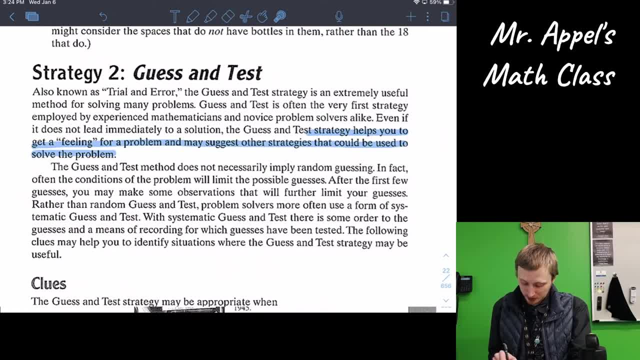 the form of systematic guess and test. With systematic guess and test, there is some order to the guesses and a means of recording for which guesses have been tested. The following clues may be: may help you to identify situations where guess and test strategy may be useful. 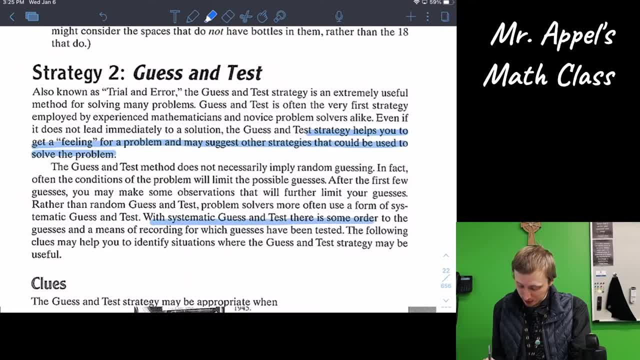 And let me just highlight that again, Systematic guessing and testing has order and recording what has been tested, So you don't test the same thing again. so you can see, maybe you want to start spacing out your test, Maybe you want to try some more specific types. 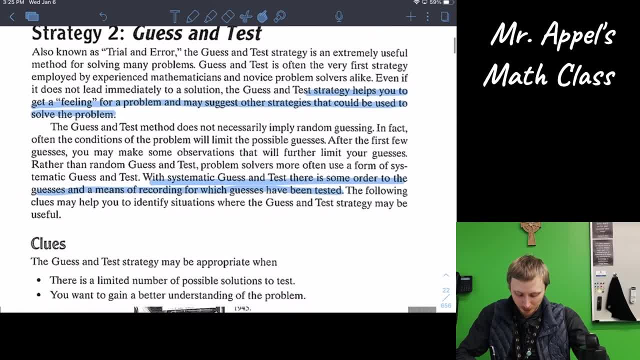 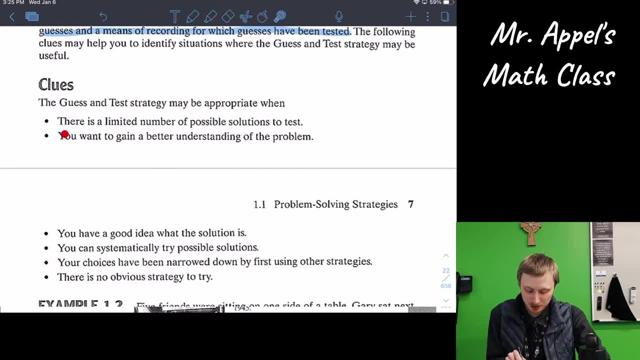 of guesses in the future. Guess and test strategy may be appropriate when- Here are the clues- There is a limited number of possible solutions to test. You want to gain a better understanding of the problem. You have a good idea what the solution is. 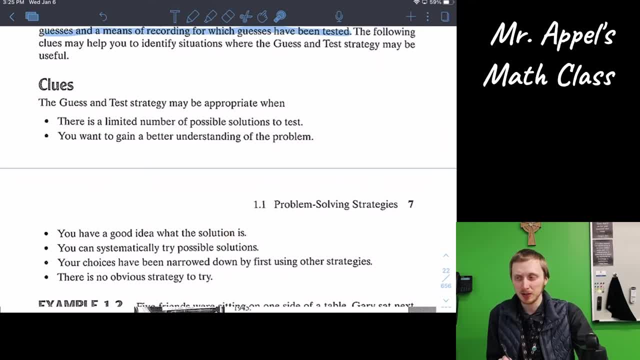 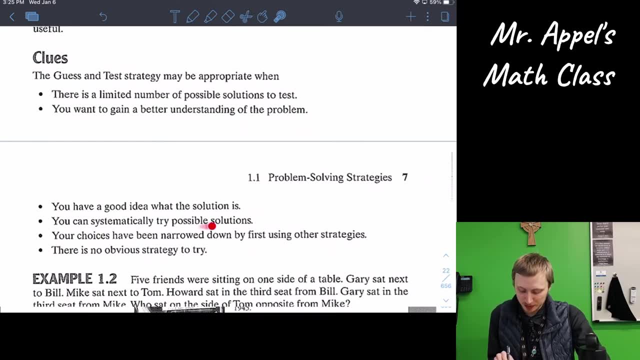 So not that you think you already know, but you have a feeling that says, ooh, I bet this number is really good. here You can systematically try possible solutions. Your choices have been narrowed down by first using other strategies or even the problem itself. 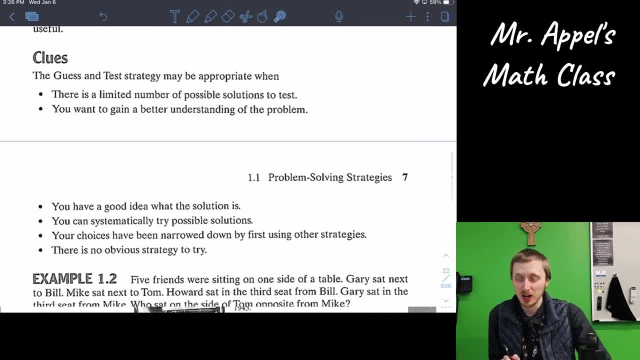 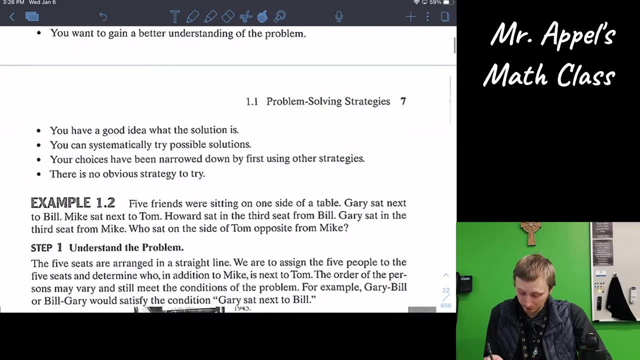 Or if there is no obvious strategy to try. If nothing else seems helpful, then at least start here, because it will do something. So, for example, five friends were sitting on one side of a table. Gary sat next to Bill, Mike sat next to Tom. 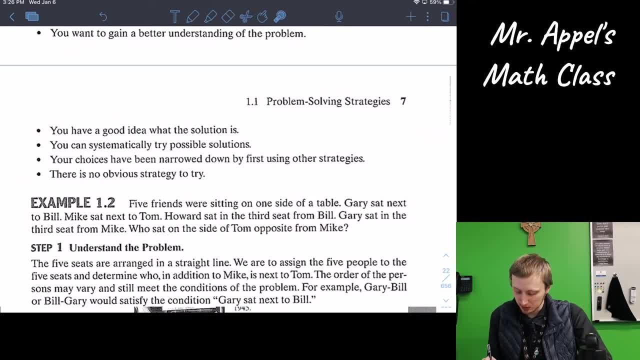 Howard sat in the third seat from Bill. Gary sat in the third seat from Mike, Who sat on the side of Tom, opposite from Mike. Okay, so we could visually start putting these together, but since we don't know where to begin with, who's sitting where? 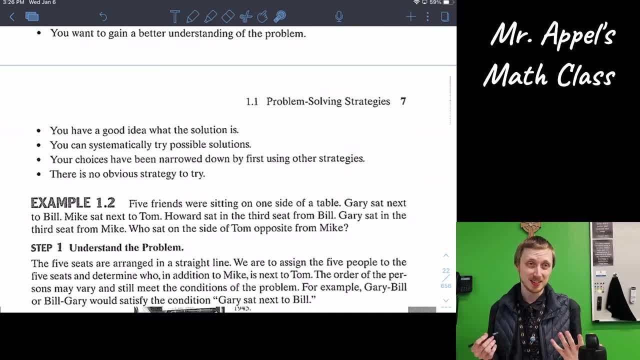 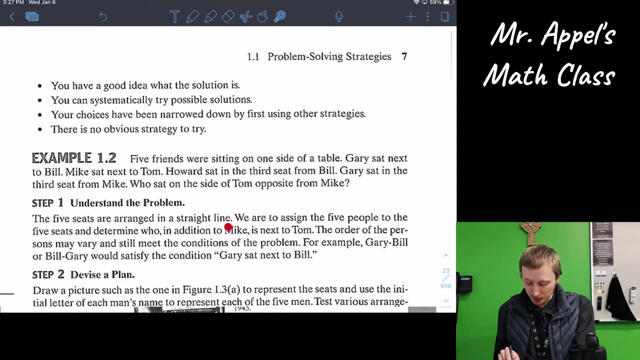 this sounds like a good place to start with a test and see. maybe we will have to arrange, because there's only five seats, There's not that many total combinations. to try. Step one, understanding the problem, The five seats are arranged in a straight line. 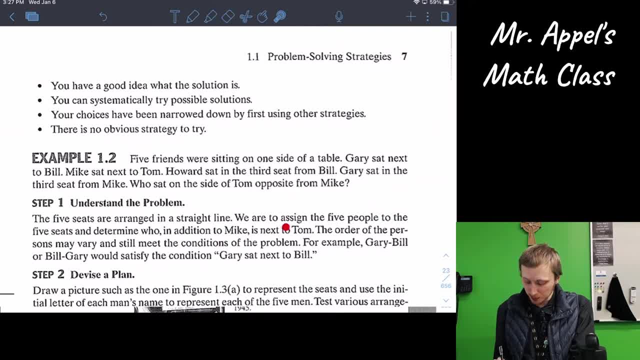 They're all on the same side of the table. We are to assign the five people to the five seats and determine who, in addition to Mike, is next to Tom. The order of the persons may vary and still meet the conditions of the problem. 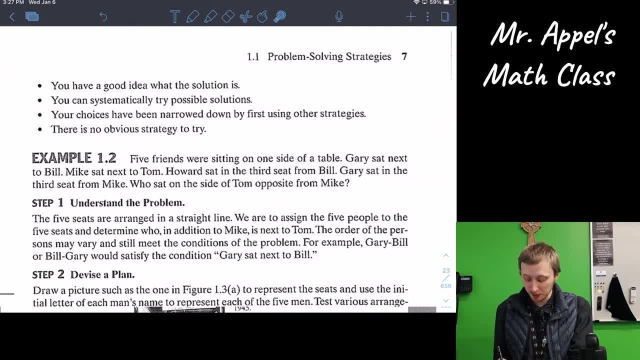 We only care about who is next to Tom besides Mike. The rest of the people where they're seated is not part of that consideration. It might help us get there, but it's not important. For example, Gary-Bill or Bill-Gary would satisfy the condition. Gary sat next to Bill. 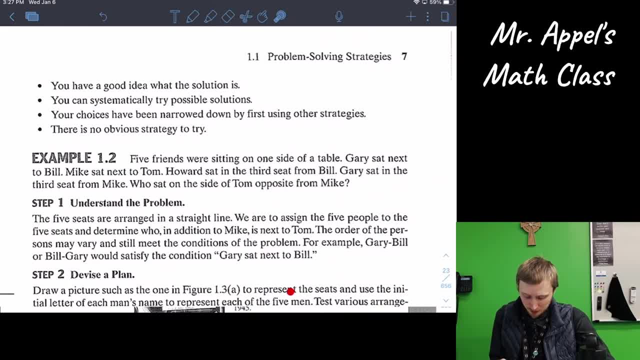 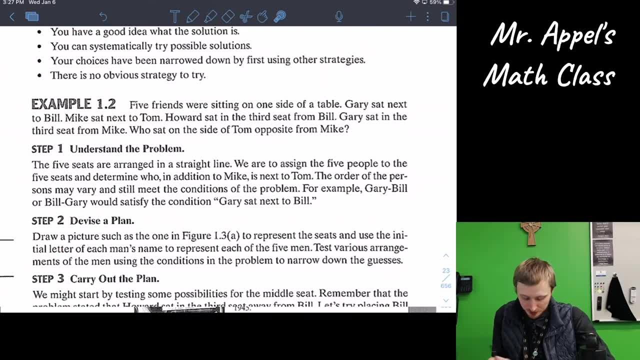 Which side is not specified. So our plan is to draw a picture such as the one in Figure 1-3 to represent the seats and use the initial letter of each man's name to represent each of the five men. We will test various arrangements of the men. 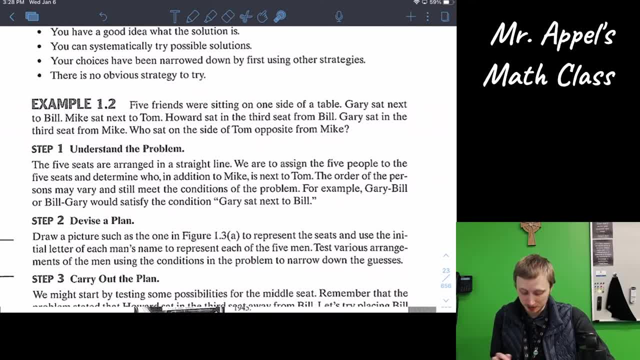 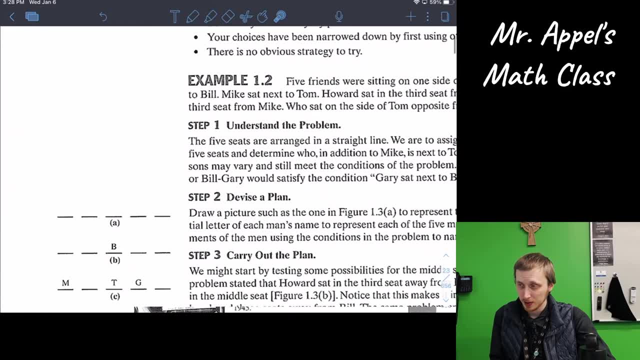 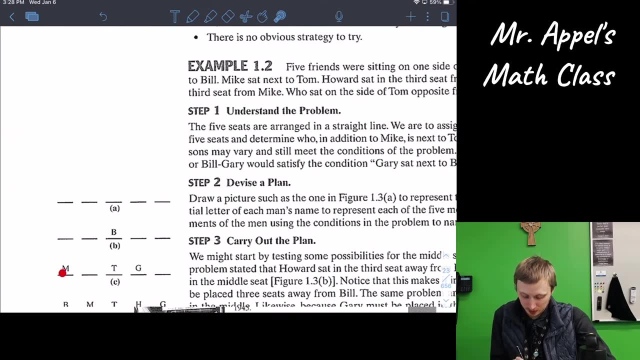 using the conditions in the problem to narrow down the guesses. So here we have five blank seats. We start systematically adding each clue. We'll put Bill in somewhere. Will that work? How about Mike goes here, Tom, and what was G for Gary? 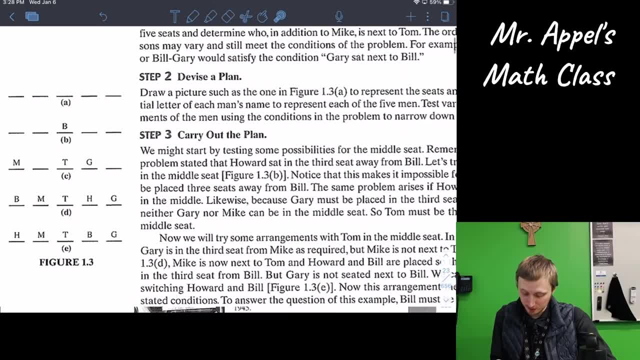 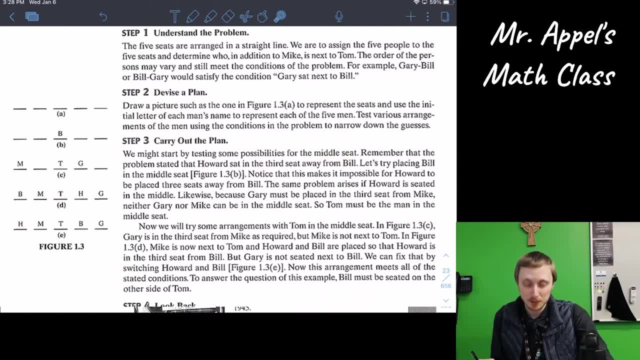 All right, that is the carrying out of the plan. So we might start by testing some possibilities for the middle seat, because that seems to have the most options. Remember that the problem stated that Howard sat in the third seat, away from Bill. Let's try placing Bill in the middle seat. 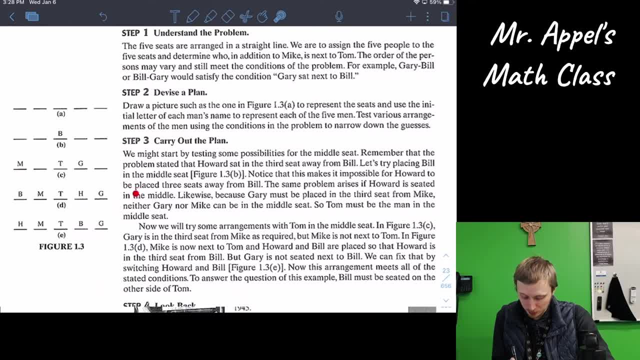 Notice that it makes it impossible for Howard to be placed three seats away from Bill From here: one, two, three. Oh wait, there's no chair there, So that won't work. Same problem arises if Howard is seated in the middle. 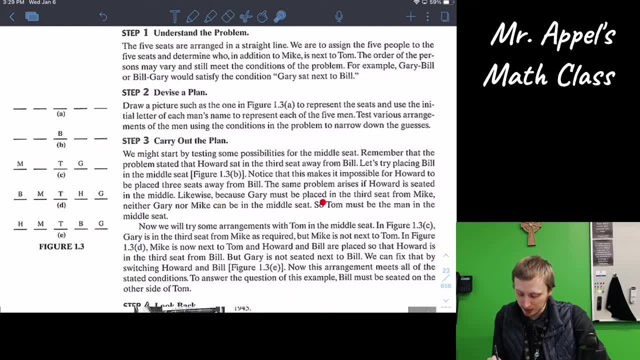 Likewise, because Gary must be placed in the third seat from Mike. neither Gary nor Mike can be in the middle seat. That really narrows it down now, doesn't it? It must be Tom, It must be the man in the middle seat. 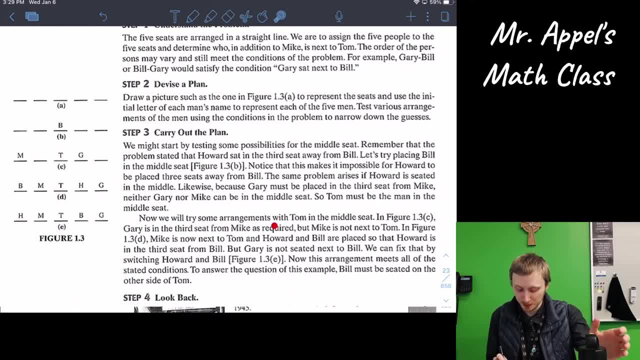 So that's why we filled in Tom there. Now we will try some arrangements with Tom in the middle. In Figure 1-3-C, Gary is in the third seat from Mike, as required, but Mike is not next to Tom. So from Mike one, two, three to Gary. 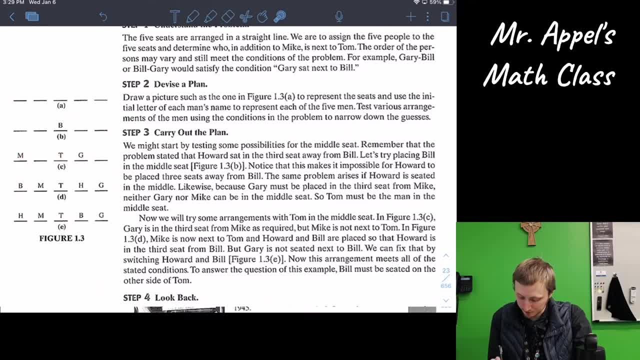 but it says Mike is supposed to be next to Tom and that didn't happen. So in Figure 1-3-D we've switched him. Mike is now next to Tom and Howard and Bill are placed so that Howard is in the third seat from Bill. 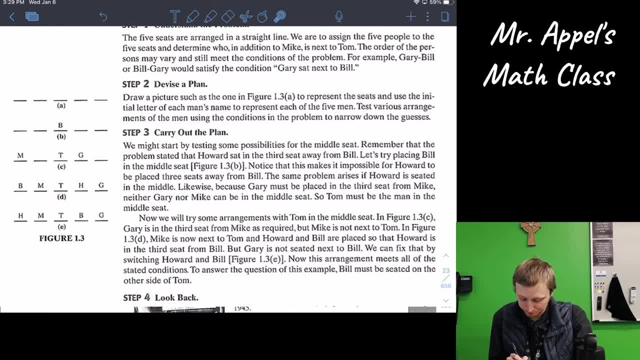 Bill. one, two, three. there's Howard, But Gary is not seated next to Bill. Gary and Bill here, so that didn't work. So we can change that. We can fix that by switching Howard and Bill Didn't say where- just as long as they're three seats away. 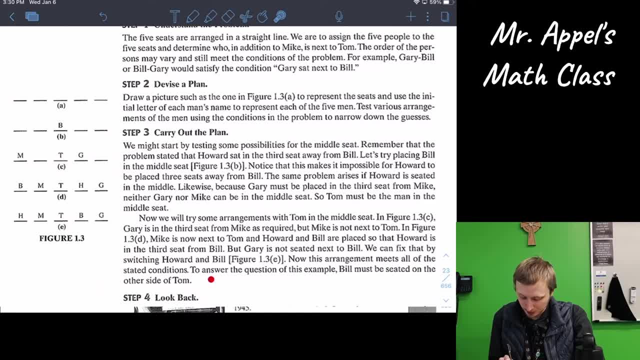 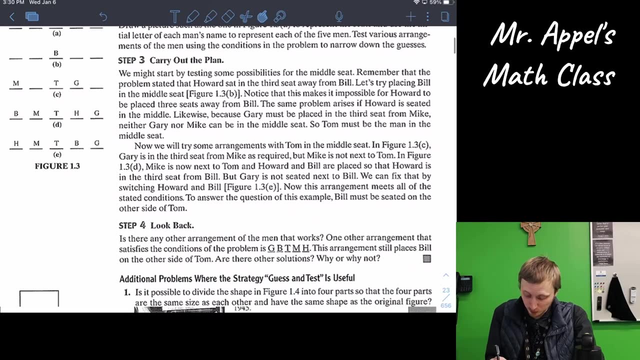 Now, this arrangement meets all of the stated conditions. to answer the question from the example, Bill must be seated on the other side of Tom. right, We want to know who sat next to Tom besides Mike, and that would leave us with Bill. So, looking back, Step 4,. 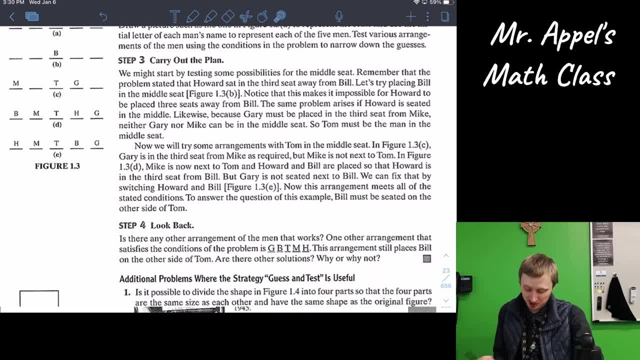 is there any other arrangement of the men that works? One other arrangement that satisfied the condition is G-B-T-M-H, G-B-T-M-H, G-B-T-M-H. That's just the same thing, except backwards right. This arrangement still places Bill. 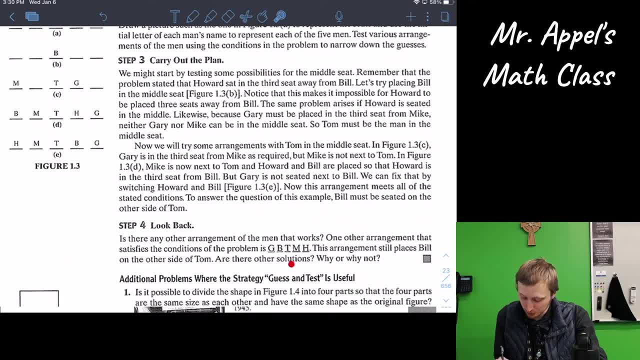 on the other side of Tom. Are there other solutions? Why or why not? That's an interesting thing to consider, And if you've gotten this far and you had your own solution, check: is your solution the same as this one or did you find something different? 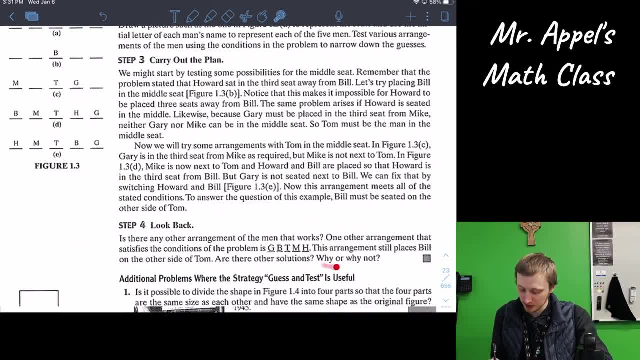 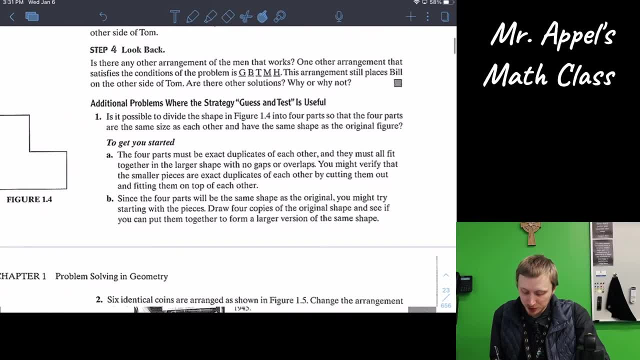 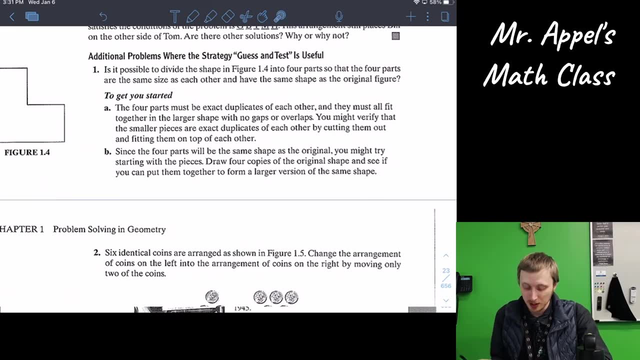 If you didn't, is it possible to find something different? Yeah, try answering that question. Go one beyond. A couple additional problems for you to try. Go ahead and read through. pause. read through these. Give them a shot. This one has to do with dividing up this L shape. 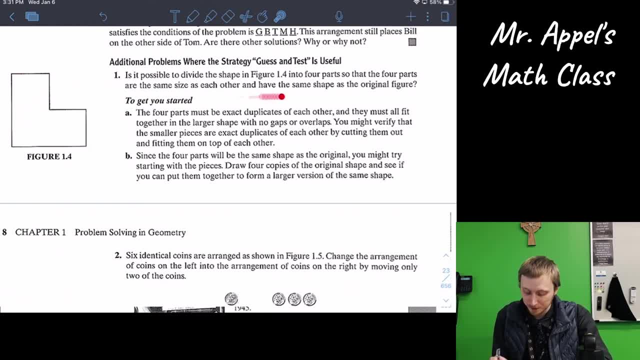 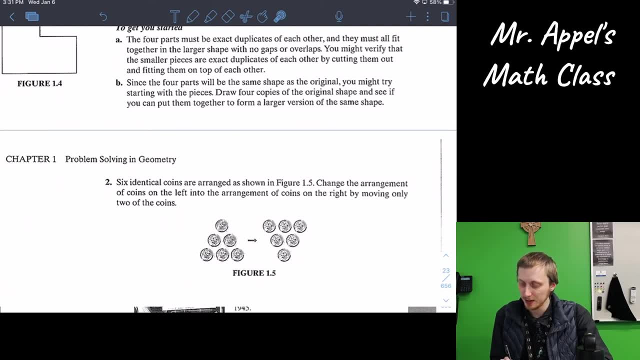 into subsequent smaller L shapes. And the second one has to do with rearranging coins in one triangle into another. I would highly recommend going and getting some coins or buttons or other small objects and trying this physically out in space. It will save you a lot of paper. 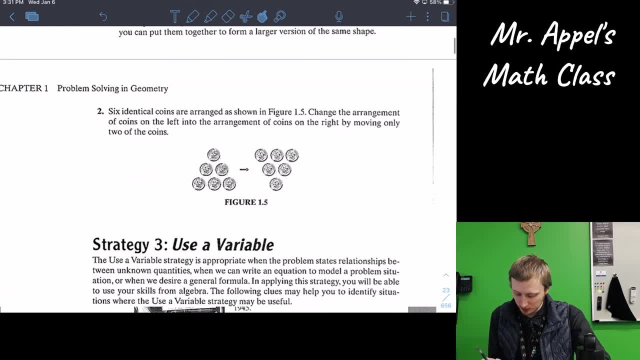 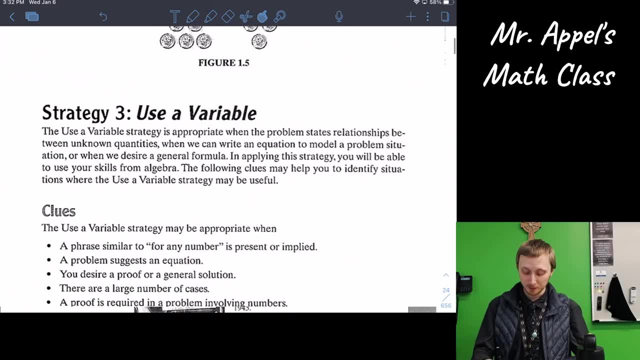 All right, now that you are done with those, let's finish off with strategy number three: Use a variable. The use of variable strategy is appropriate when the problem states relationships between unknown quantities. Relationships between unknown quantities. That sounds like algebra to me. 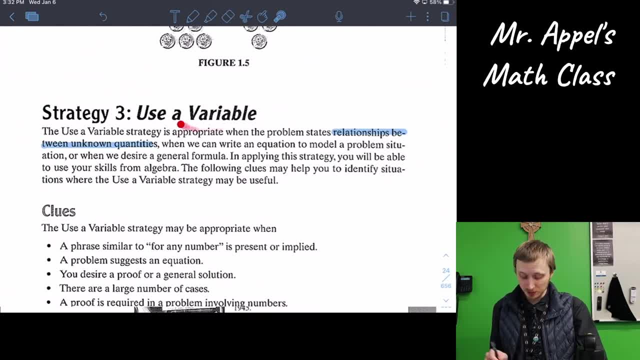 which is what a lot of algebra contains. using of variables. When we can write an equation to model a problem situation, that's a good one. write an equation, or when we desire a general formula. In applying this strategy, you will be able to use your skills. 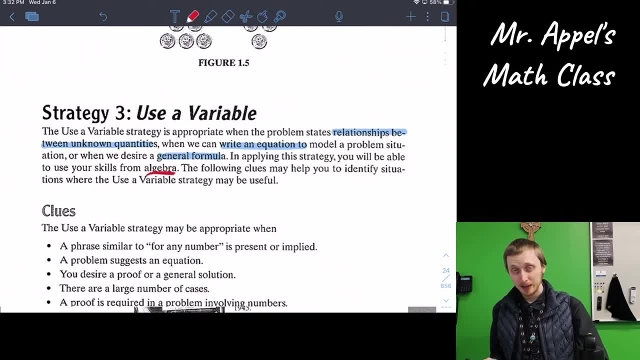 from algebra right. Once you get that final algebraic equation, it no longer becomes a problem. it turns into just an algebra exercise. The following clues may help you identify situations where use a variable may be useful. A phrase similar to for any number. 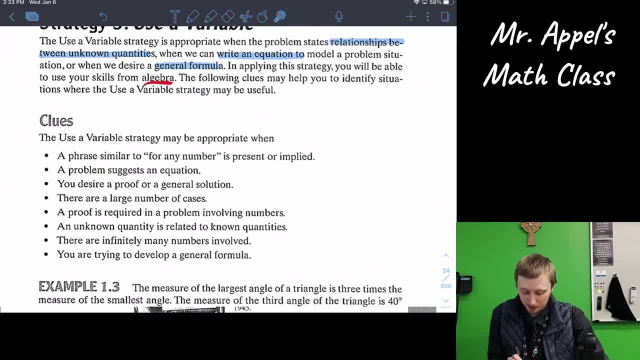 is present or implied. A problem suggests an equation. You desire a proof or a general solution. There are a large number of cases. Contrast that to the prior one with guess and test, where there's only a few possible cases. A proof is required in a problem involving numbers. 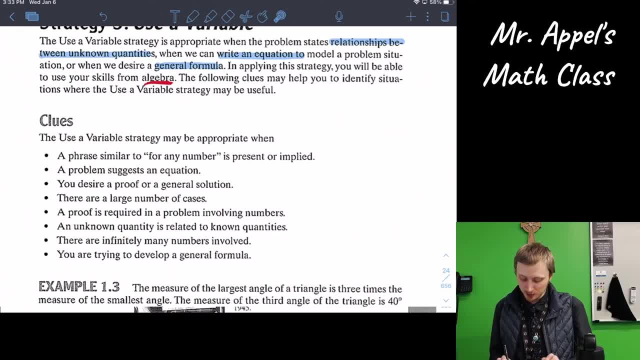 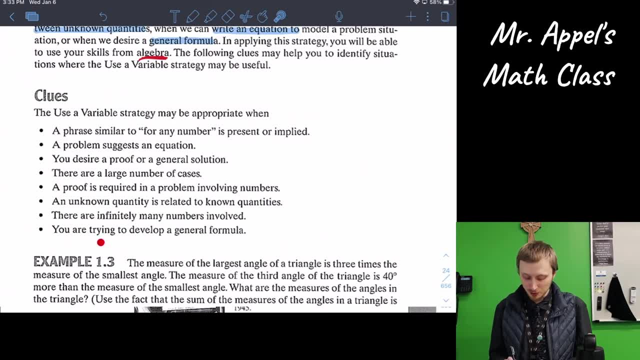 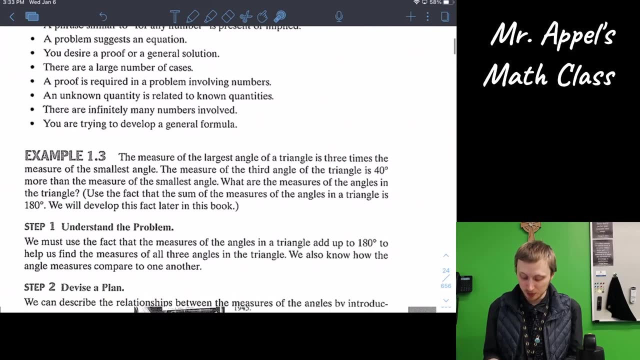 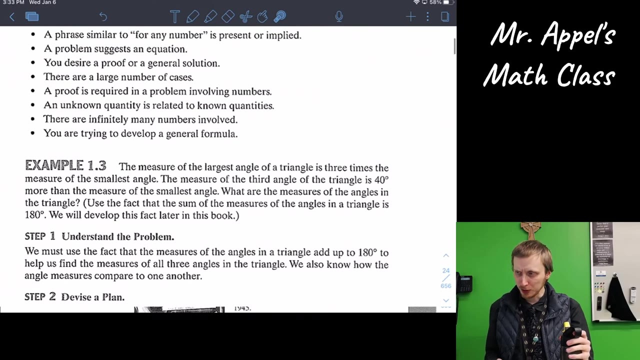 An unknown quantity is related to known quantities. There are infinitely many numbers involved, Or you are trying to develop a general formula, So let's take a look at an example of using a variable in action. I don't want to give too much away. 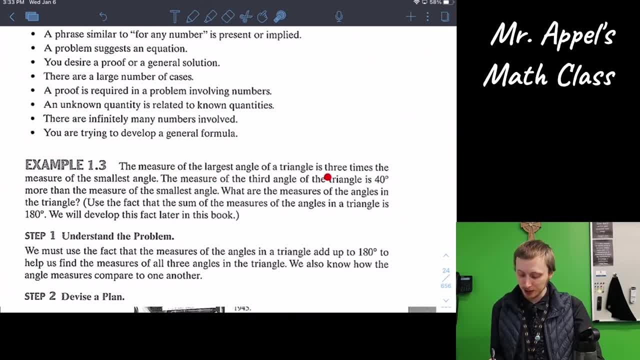 Here we go. The measure of the largest angle of a triangle is three times the measure of the smallest angle Number is three times something else That sounds like a relationship. The measure of the third angle of the triangle is 40 degrees more. 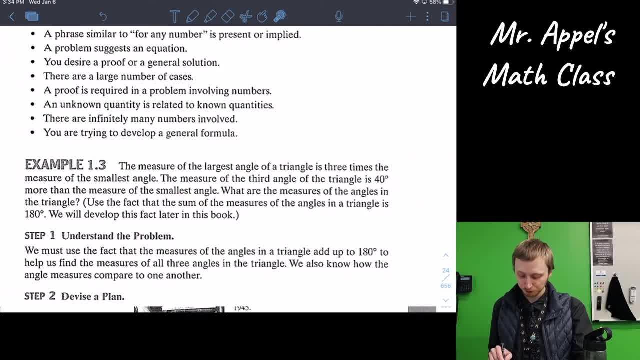 Then the measure of the smallest angle. What are the measures of the angles in the triangle? Use the fact that the sum of the measures of the angles in a triangle is 180 degrees. We will develop this fact later in the book. So there's a little geometry fact for you. 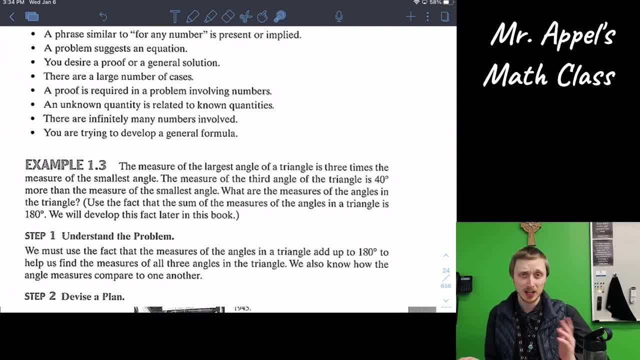 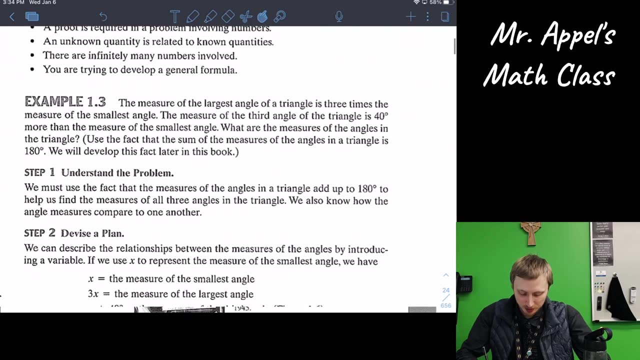 necessary for solving this. Go ahead and pause now. Try this problem out for yourself. Give it some thought. Now that you've had a chance to consider that yourself, let's see the solution process. In understanding the problem, we must use the fact that the measures 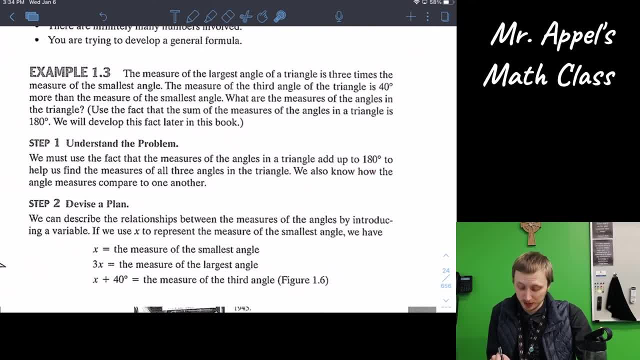 of the angles in a triangle add up to 180 degrees. There's a reason they gave that to us. Anything in parentheses in a problem is a good hint. that it's a hint and shouldn't be ignored. to help us find the measures of all three angles in the triangle: 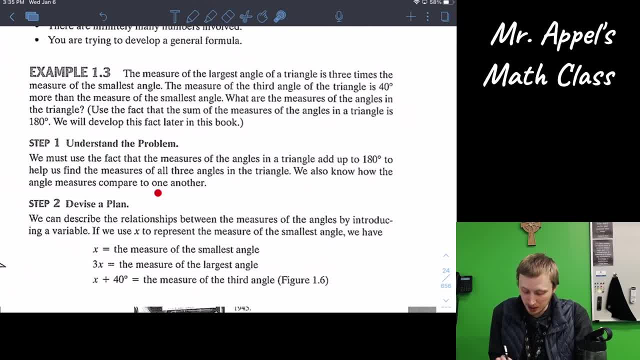 We also know how the angle measures compare to one another, So we can describe in creating our plan here we can describe the relationships between the measures of the angles by introducing a variable, And this just lets us write these out in a mathematical context much easier. 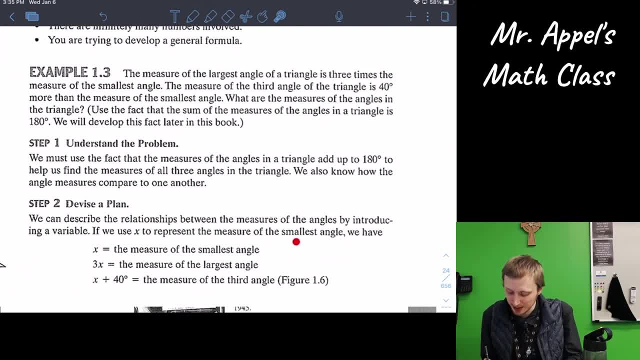 If we use x to represent the measure of the smallest angle, it could have been any. So x is smallest somewhat arbitrarily here, But I would recommend smallest because it said one thing is three times measure of the smallest angle. Right, If x is the smallest. 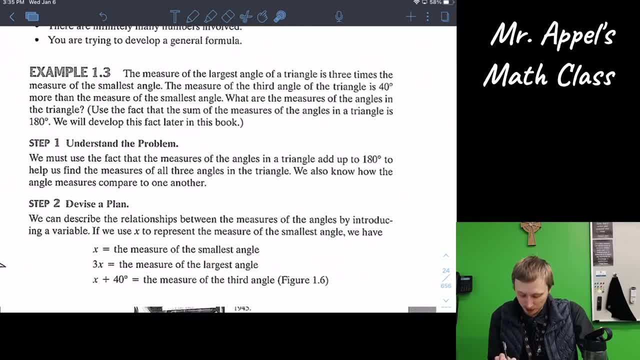 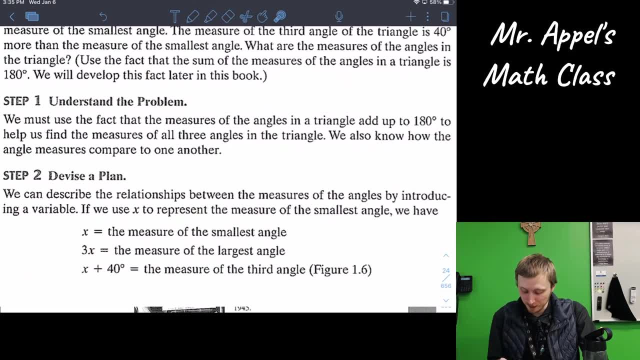 then you have: 3x is the measure of the largest. If I reversed that and made x be the largest, I'd then have to use one-third, And I know a lot of you will rather avoid fractions. And then, finally, the third angle, right. 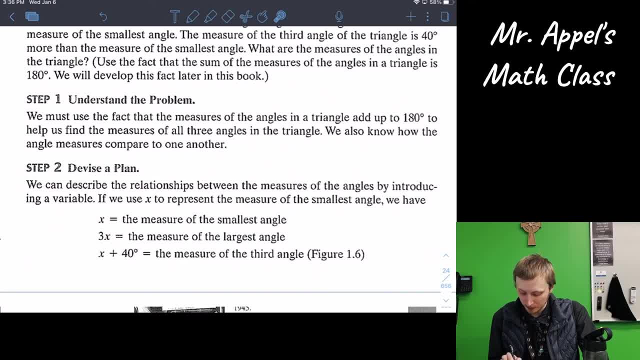 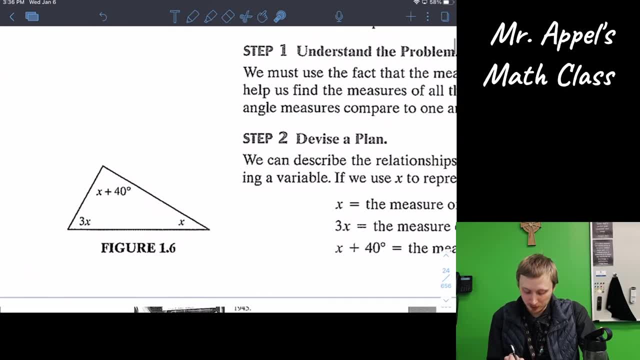 You've got the smallest, the biggest and the one in the middle. The third angle is 40 more than the smallest, So x plus 40 equals the third angle. We've got that in picture form right here: our triangle: small, medium and. 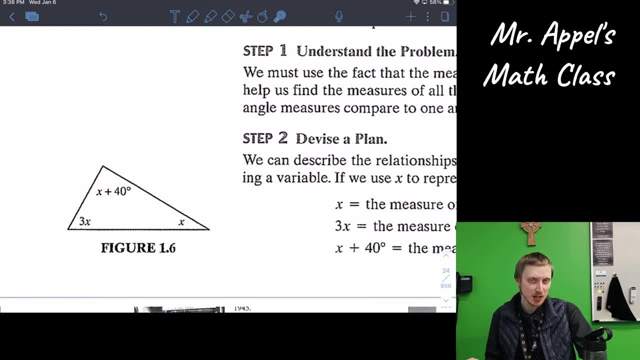 This doesn't look like the medium. Clearly the figure is not drawn to scale, but we're just whipping up a solution here. I'm not building a bridge out of it, so the scale does not matter as long as we can reference which angle is which. 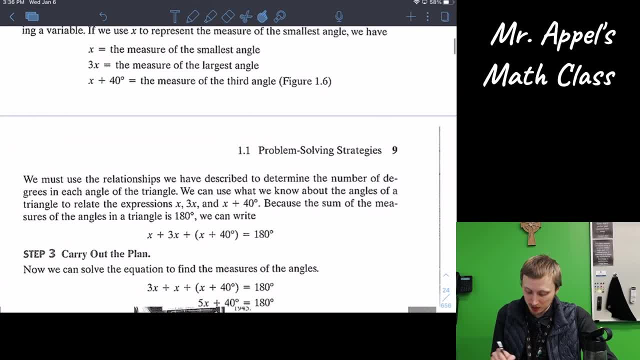 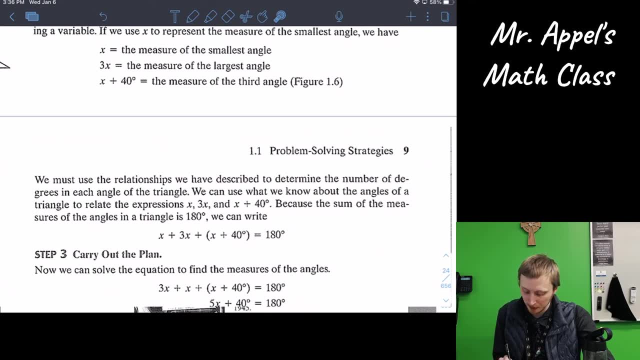 So we must use the relationships we have described to determine the number of degrees in each angle of the triangle. We can use what we know about the angles of a triangle to relate the expressions x, 3x and x plus 40.. 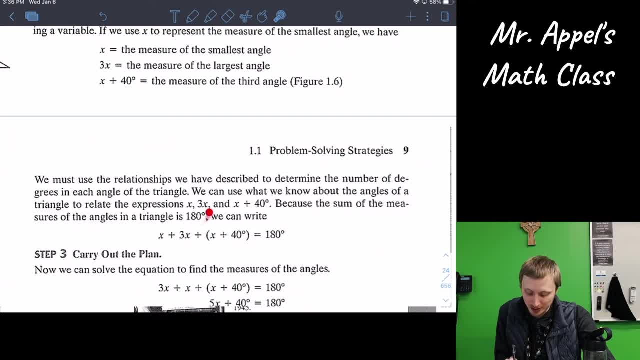 Because the sum of the measures of the angles in a triangle is 180, we can write- here's our equation: add all three together: x plus 3x plus x plus 40 equals 180. And carrying out the plan is just solving the equation. 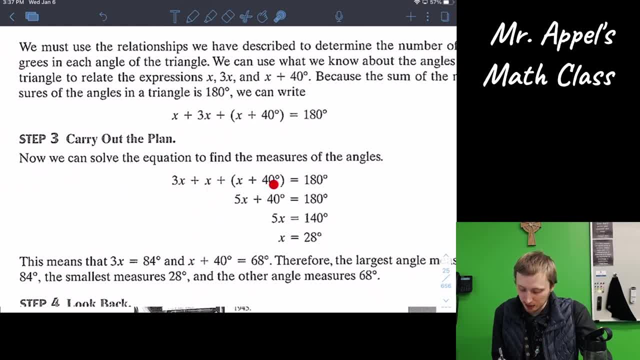 Solve the equation to find the measure. So we will combine like terms. thus: so subtract the 40 from both sides and then divide by 5 to get x equal to 28 degrees. We can substitute that back in to find the other measures. 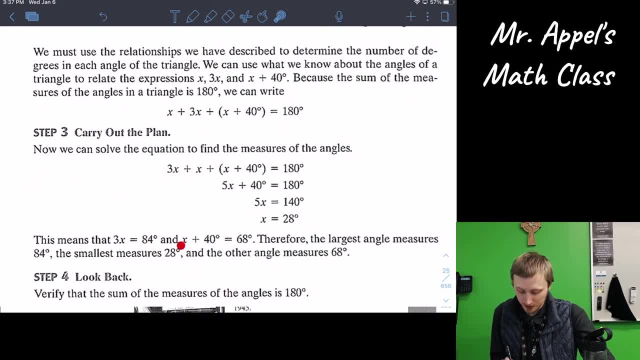 So that means 3x is 84 degrees and the x plus 40 is 68 degrees. therefore the largest angle measures 84 degrees, smallest measures 28, and the other 68, respectively. Looking back, we can verify that the sum 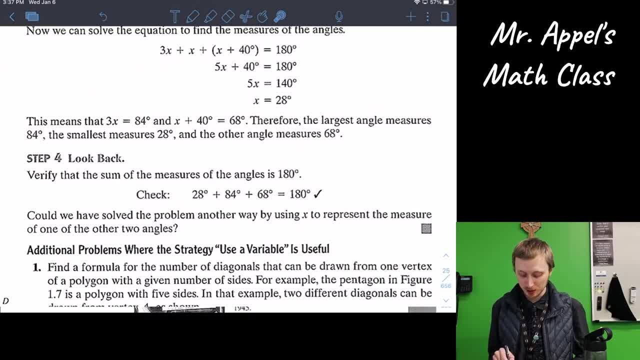 of the measures of the angles is 180.. So check with those numbers: 28 plus 84 plus 68 is in fact 180.. Yes, it works. Could we have solved the problem another way, By using x to represent the measure? 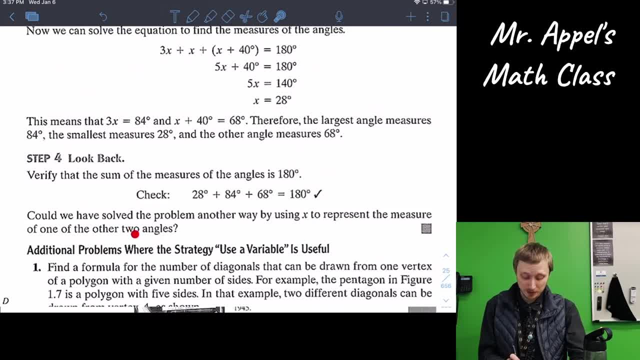 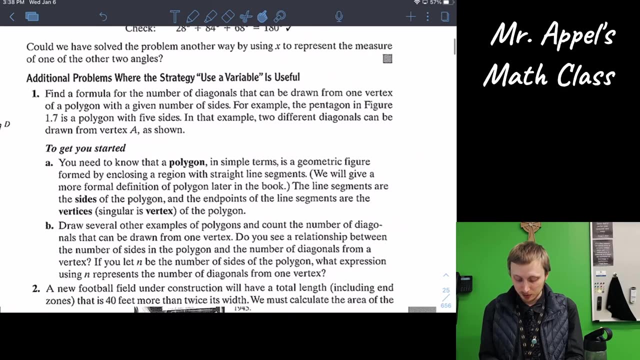 of one of the other two angles. I kind of talked about that when we were setting it up. So absolutely, you could have done that, It just might not have looked as pretty. And then finally, here are some additional problems where using a variable might be useful. 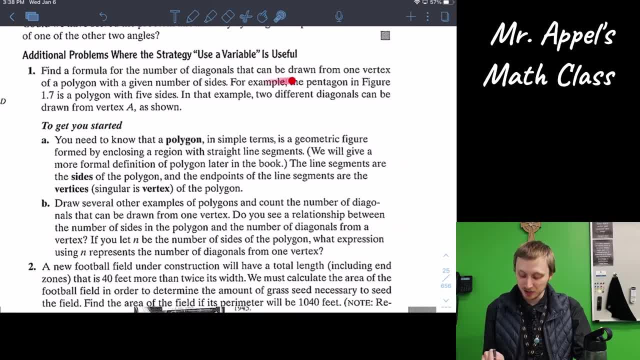 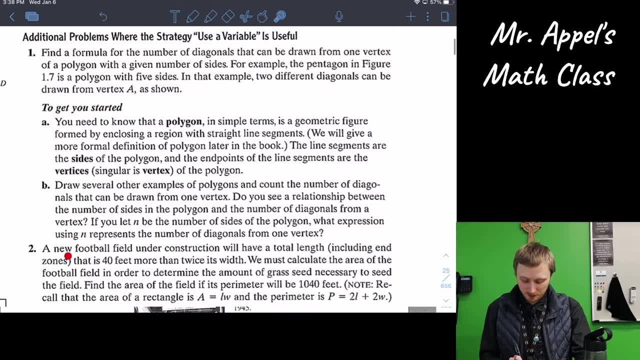 Here you're going to find the formula for diagonals in a polygon classic geometry situation, And the second one involves a football field. We have some descriptions of how its widths and lengths compare, but we don't have the exact numbers and we need to work that out. 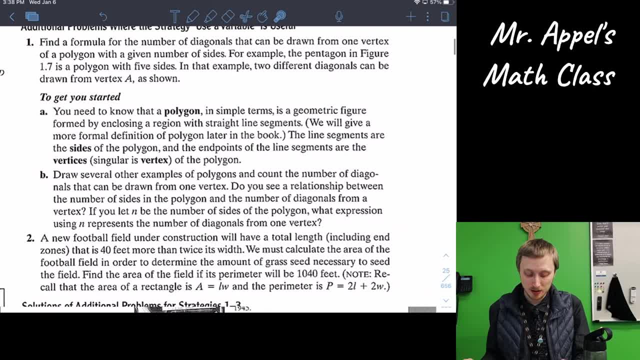 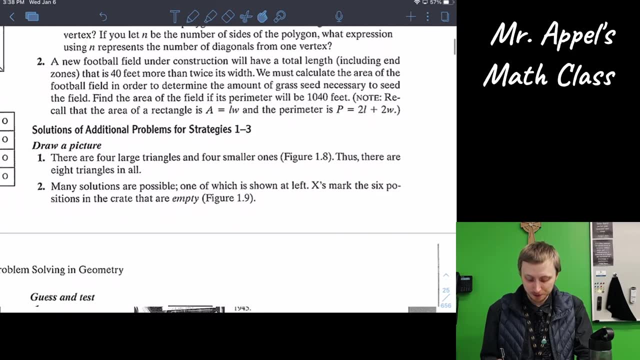 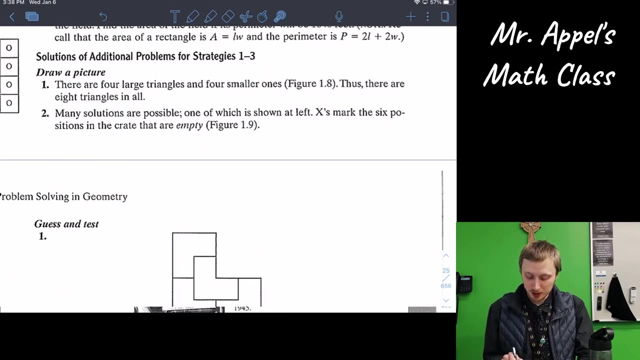 So go ahead and pause the video there and give those a shot. All done, Okay, good, because I'm going to spoil it for you. Here we have the solutions for the problems. There are four large triangles and four smaller ones, as we can see. 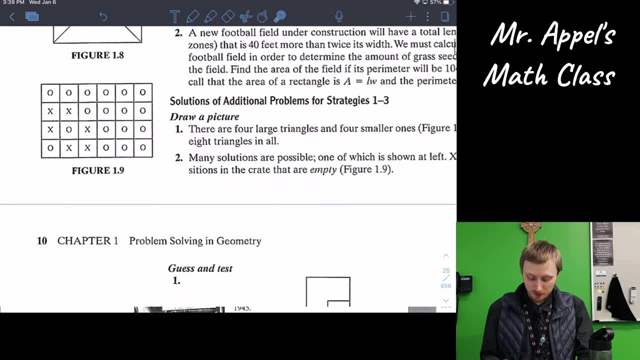 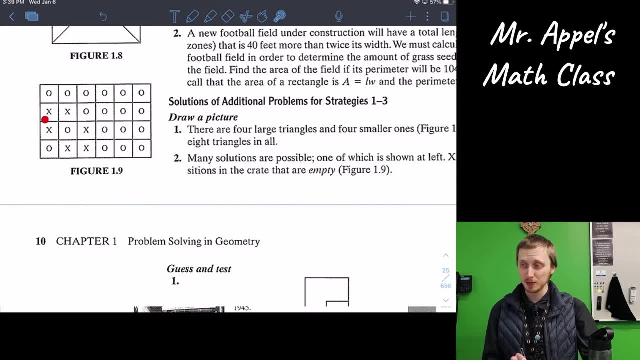 from this picture here For draw picture number two. there's many solutions possible. Here is one where the circles represent a bottle and the Xs represent an empty space. But the key to this is this little L shape of empty spaces. here You're going to have to have those. 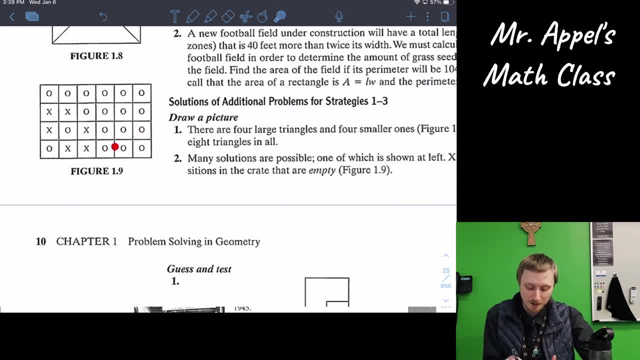 associated with one another. Of course, they could go on: either half of the milk crate or, instead of the lower portion, they could be up here, But you're going to need these kinds of shapes together, Speaking of L shapes for the guessing test. 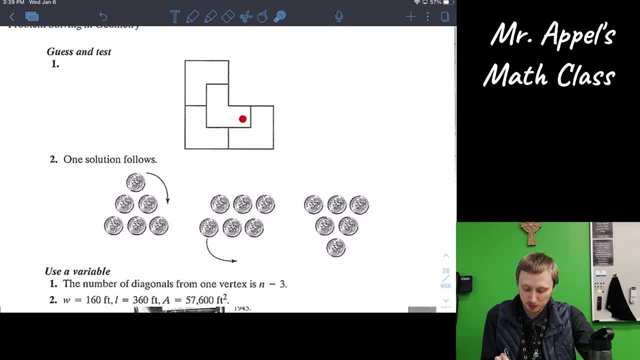 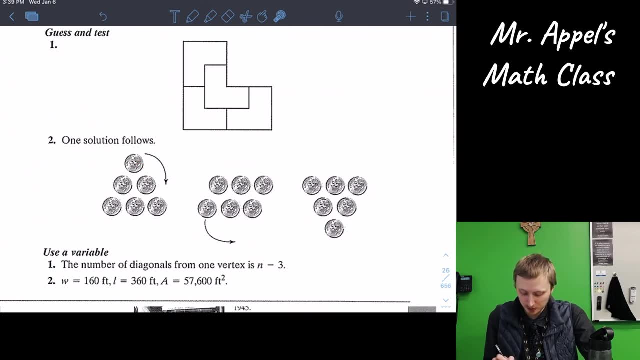 your four little Ls should be arranged thusly. And for moving the coins, it doesn't matter which end you start with, but take one end, move it down to a side there, and then take the other and move it as the tip. 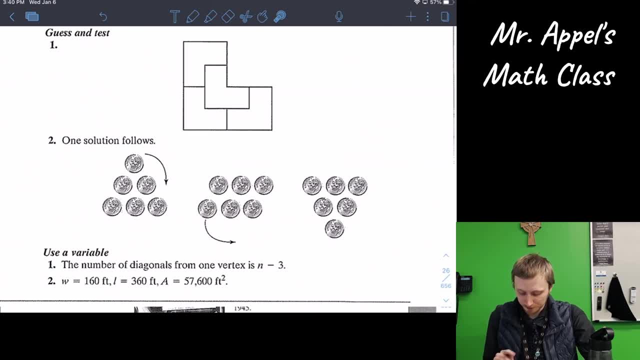 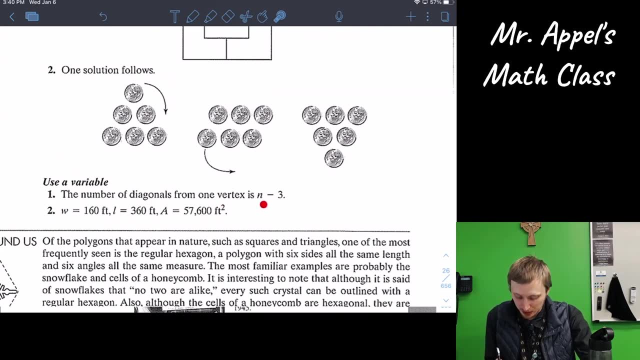 on the bottom here, And for using a variable, the number of diagonals from one vertex is n minus 3.. And for the football field the width is 160 feet. length, 360 feet. total area: 57,600 feet square. 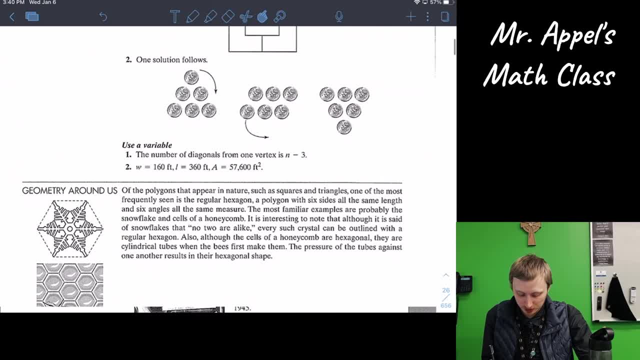 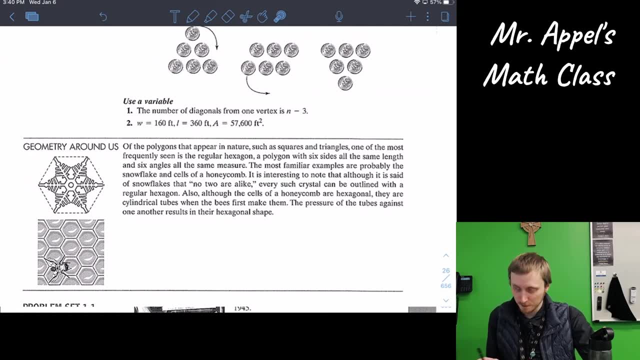 And finally, to top it off, we've got a little bit of geometry all around us. This is a nice little friendly ending note here. Of the polygons that appear in nature, such as squares and triangles, one of the most frequently seen is the regular hexagon. 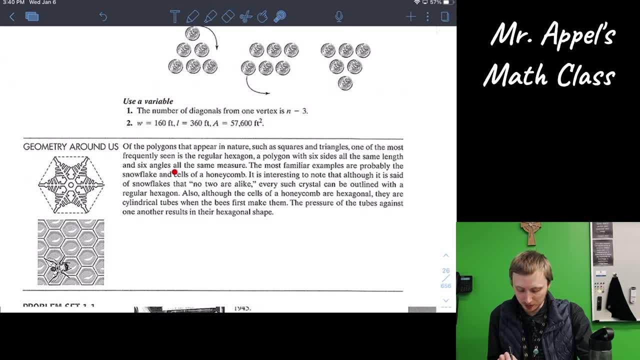 a polygon with six sides all the same length and six angles all the same measure. The most familiar examples are probably the snowflake and cells of a honeycomb. It is interesting to note that, although it is said of snowflakes that no two are alike, 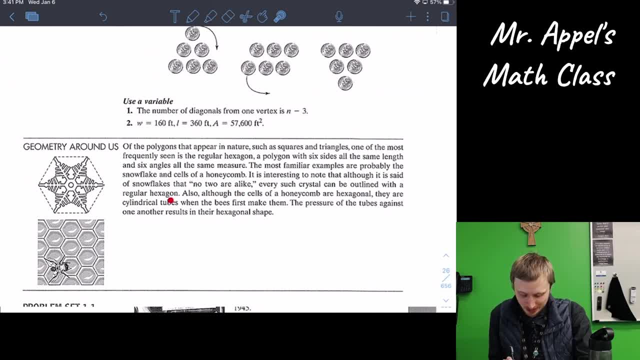 every such crystal can be outlined with a regular hexagon. I wonder why that is. Also, although the cells of a honeycomb are hexagonal, they are cylindrical tubes which the bees first make them. So they start out perfectly circular and then they kind of smoosh together. 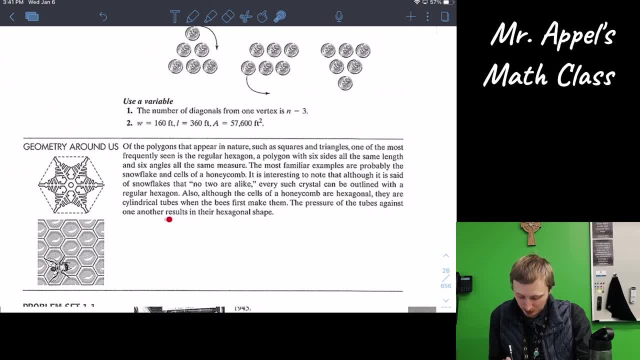 into hexagons. The pressure of the tubes against one another results in their hexagonal shape. Interesting to note. So there you go, a little bit of geometry in nature. That's going to do it for Section 1.1 of Geometry. Problem Solving Approach. 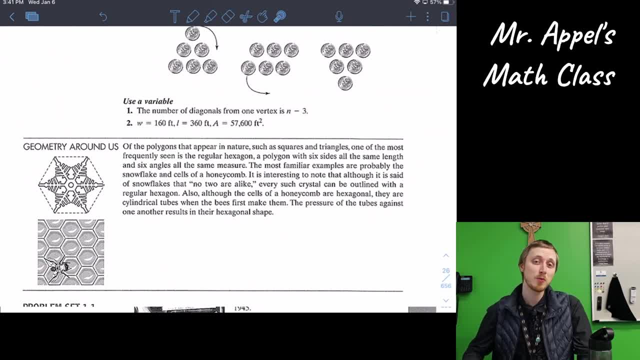 Thank you for reading along So long. farewell, enjoy the rest of your day.